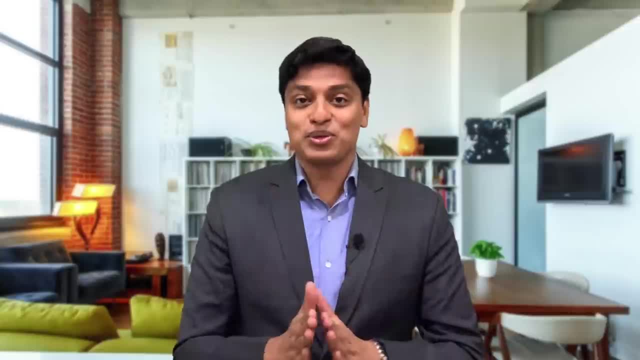 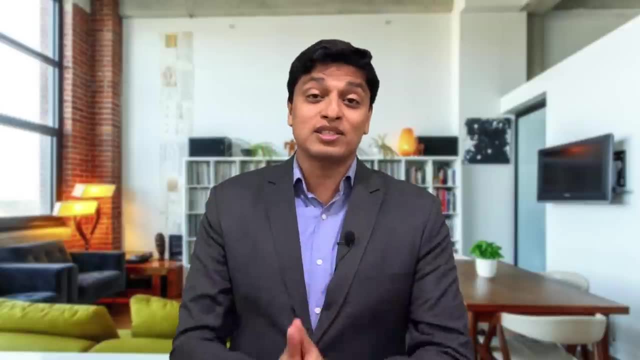 So in this video we are going to teach this to you. We are going to take up a real example of a real company from scratch and try to help you with the analysis of the income statement, the cash flows and the balance sheet. This is going to be a detailed video. 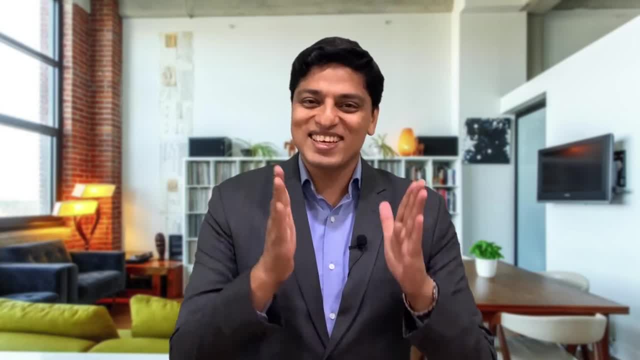 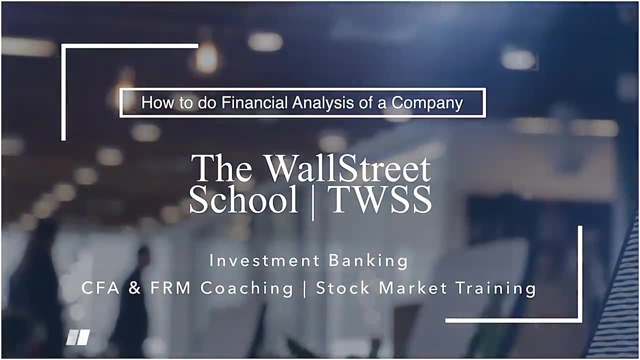 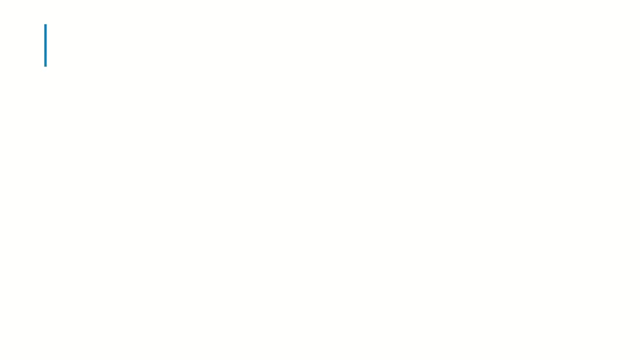 so please do not skip any part of it. Let's get started. Hello everyone, welcome back to the channel. So in this video we are going to learn how to do financial analysis of a company. Let me be very clear: in this video we are not going to learn how to do fundamental analysis. That's a wider term that 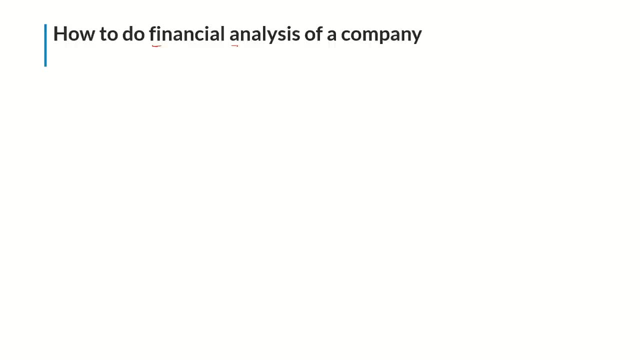 covers analysis of management, analysis of industry sector, government policy and financial statements. We are going to focus on one part of that, that is, analysis of your financial statements, profit and loss account balance sheet and your cash flow statement. It's going to be very easy. 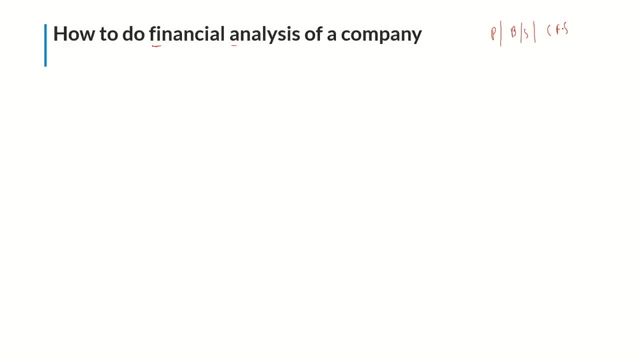 Like any person who understands these basic terms like capital, profits and all, would be able to do that. But before we move ahead, let us understand a business cycle. What is it? how a business generates money and how it put backs the money in the hands of providers of capital. 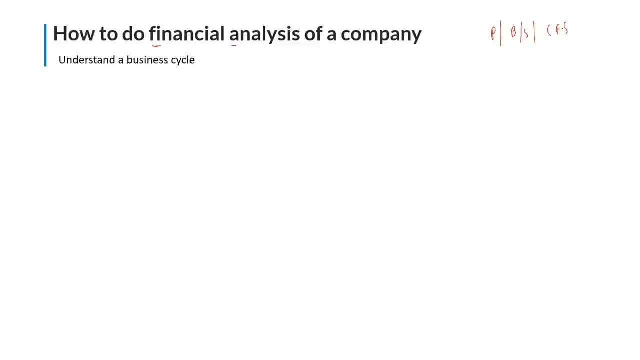 First of all, whenever I want to start any business, I need some money. that is called as capital. Either I can put in my own money, known as equity, or I can borrow it from someone else, also known as debt. Fairly easy, I need money. 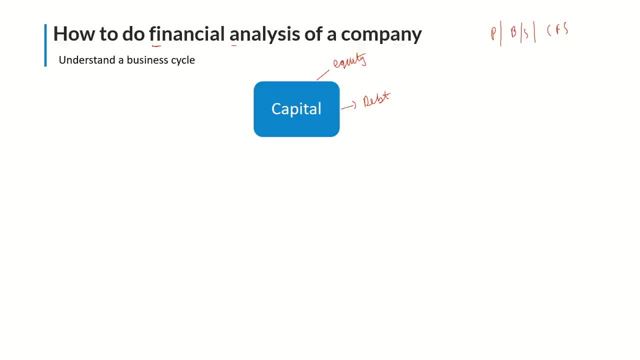 I can raise it from someone else or I can put in my own money. Once I have some money with me, I want to start a business. Suppose I want to manufacture something, I'll need some machinery, some place where I'll be putting that machinery. so land building machinery. 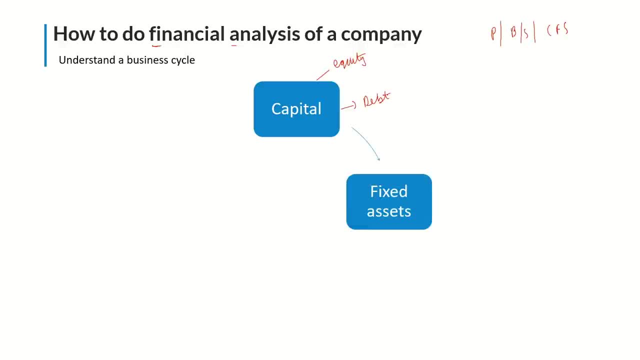 These are called as your fixed assets, that is, the instruments that will be used to produce your final goods that you will be selling in market. So these fixed assets will be used to make your final sales, and once you're able to sell some goods, you will be generating profits right. 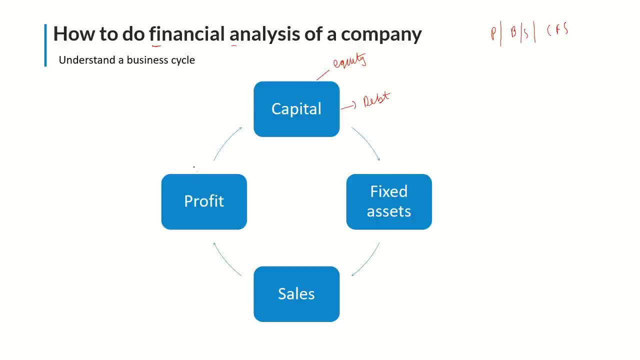 This is the entire business cycle. Once you have some profits, you can either distribute them to equity holders, also called as dividends, and you'll be paying interest of debt providers. Right. This is...this is the way. And right now the reason if a bank is doing trading and that is because these are legal businesses and a cash class business, then lets you drop some money in and move forward a direction that may require � forcémentiskхо 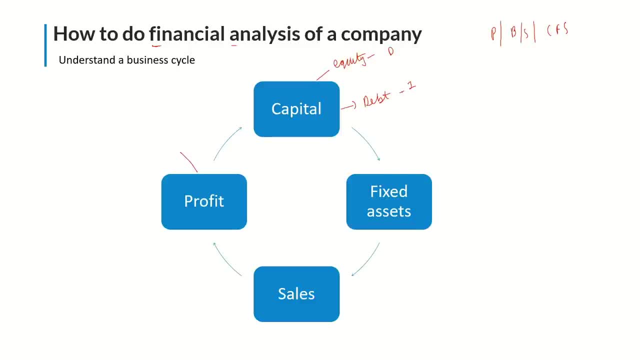 this is. this is the way, and if something extra is left, called a surplus, this will be invested in the business. then that profit will again be used to purchase new fixed assets, then to do more sales, then some more profits will be generated, and this is how business keeps. 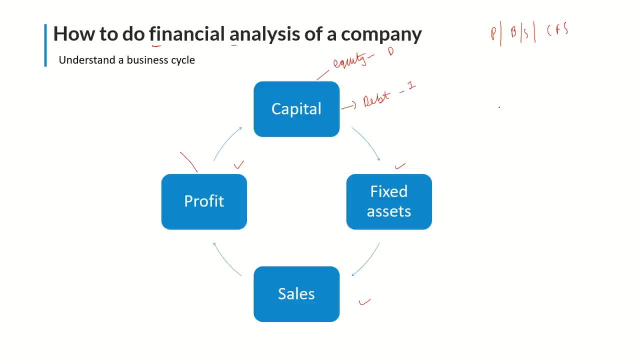 on rotating the money right and like: understand business is like a machinery. that like it's like a complicated machine. if you give it some input it will be able to generate some profits for you and you can use those profits as an inputs. so it is kind of endless loop. 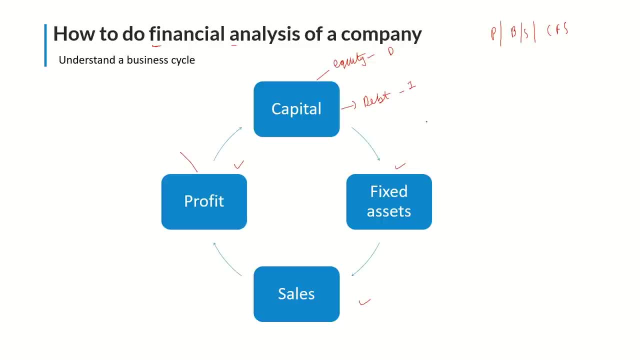 right, but you have to make sure that your machine is looped properly. it's not suffering. so that is working capital. suppose you want to purchase some raw material to manufacture your finished goods, but you don't have money for it right now. but if you don't purchase, 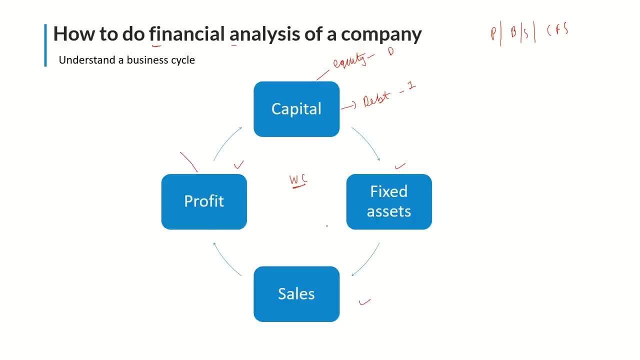 what will you sell? your business will stop doing its activities so you can get it on credit. that is your working capital. if someone wants to buy some raw material, then you can buy some raw material and then He wants material from you, your finished goods from you, and he's not able to pay you. 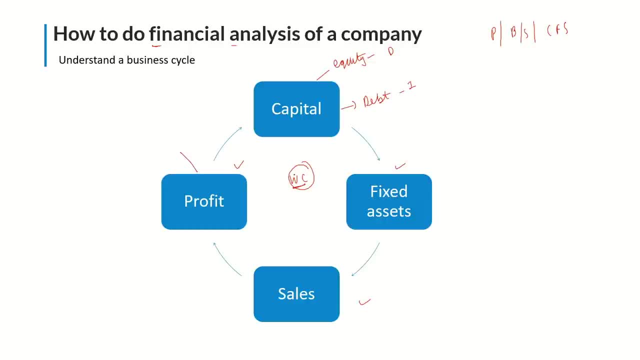 right now. Maybe he'll be able to pay you in one month. Then still, if you want to generate profits, then you can give that person something on credit. that is called as your working capital debtors, right? So working capital is kind of a loop to your machinery known as business. 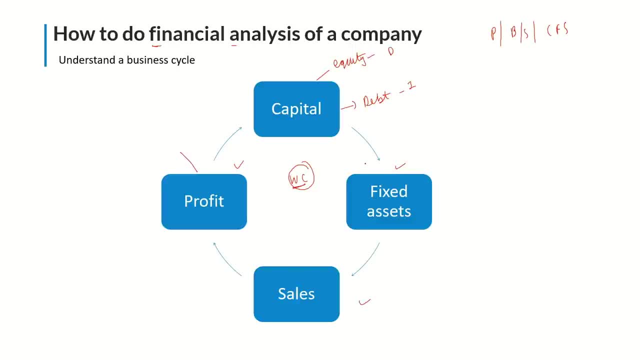 It's very simple. right Now I'll be directly jumping to my website called a screenerin- S-C-R-E-E-N-E-Rin. I'll be getting some data from that and we'll be learning how to do analysis of profit and 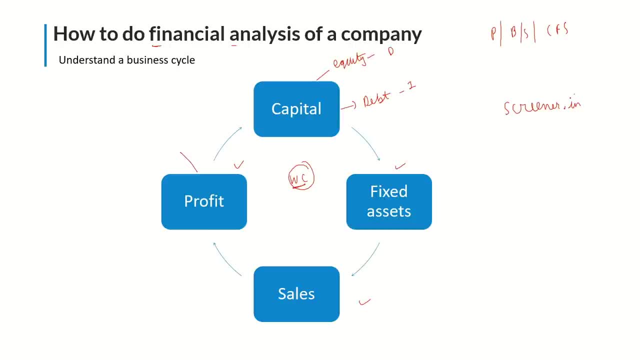 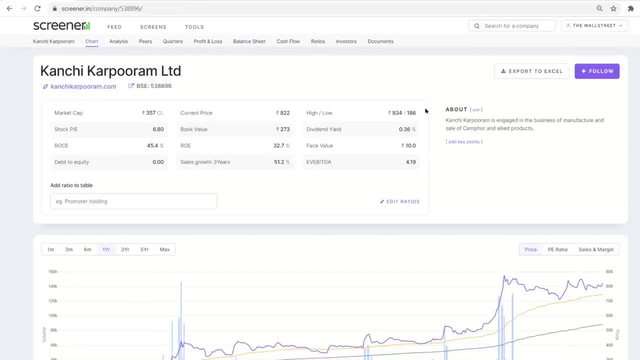 loss account balance sheet and cash flow. It's going to be very simple, Okay, so let me open Google Chrome, and this is the company that we'll be using to analyze Kachi Karpuram Limited right. You can read very briefly about it here: 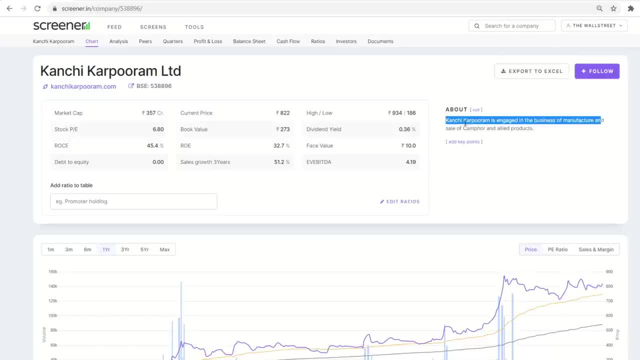 Kachi Karpuram is engaged in the business of manufacturing and sale of camphor and allied products. Okay, We are not going to read about businesses and all right. now we are just going to focus on P&L balance sheet and cash flow. 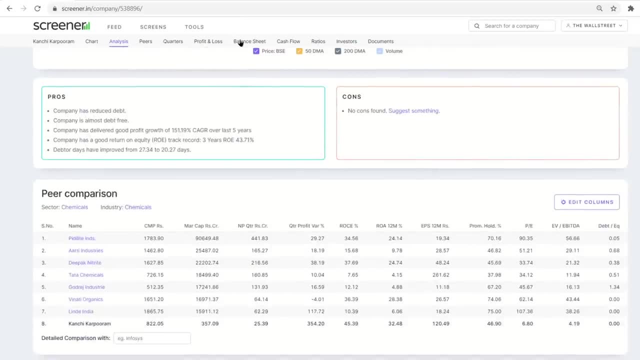 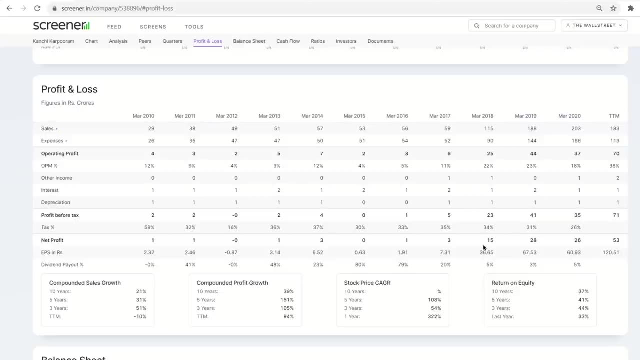 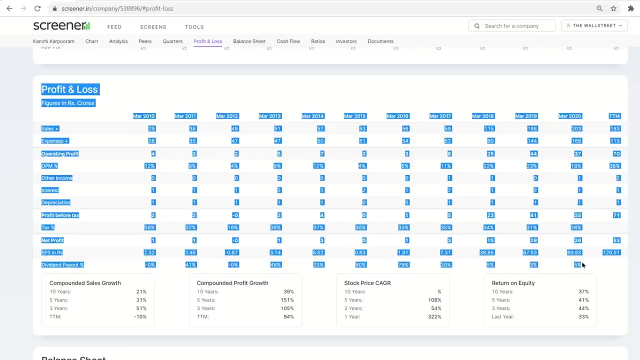 So this is the company. If you scroll down or if you can click here, it will take you to profit and loss account. See, it becomes very difficult to do some analysis on the sheet, right? So what I'll do is I'll just copy this data, I'll select it and then I'll press control. 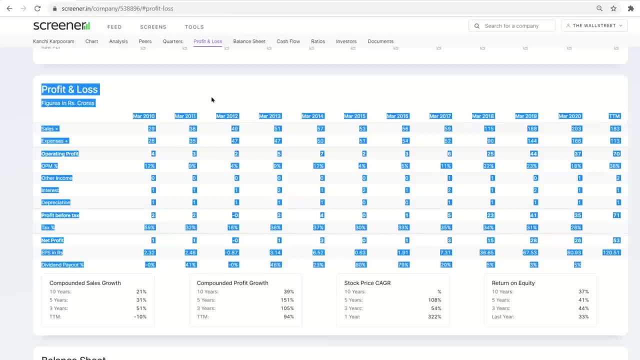 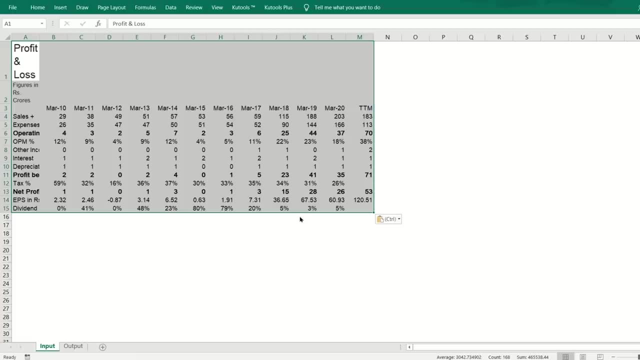 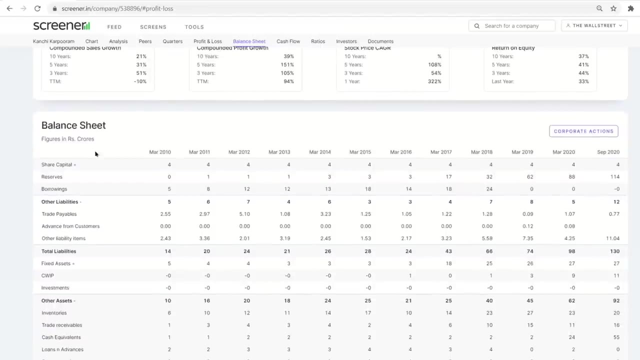 C, The entire profit and loss account is copied right. I'll just go to MsExcel and we'll paste it. simply control C, control V. Going back again to Google Chrome, here, just below their profit and loss account, You have your balance sheet. 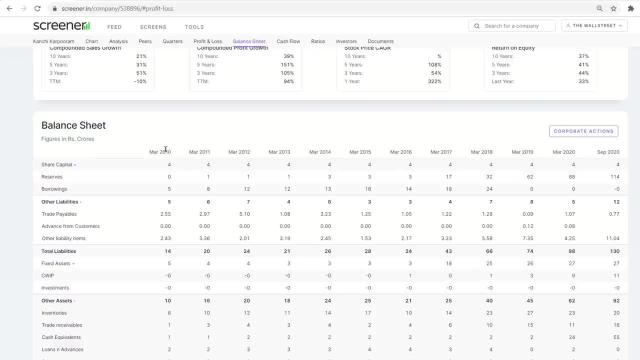 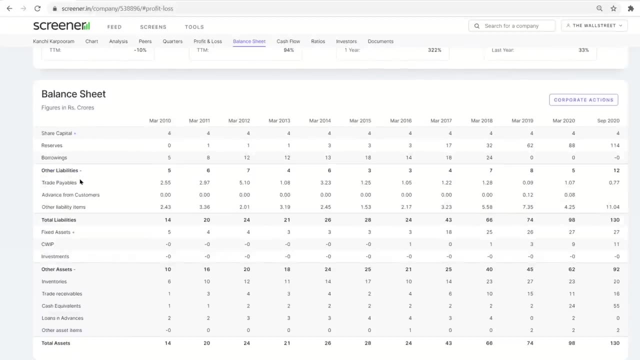 This profit and loss account is from 2010 till now. This balance sheet is also from last 10 years, So in this balance sheet I'll be just clicking on this sign: It will expand other liabilities And on This sign, it will expand other assets. right, 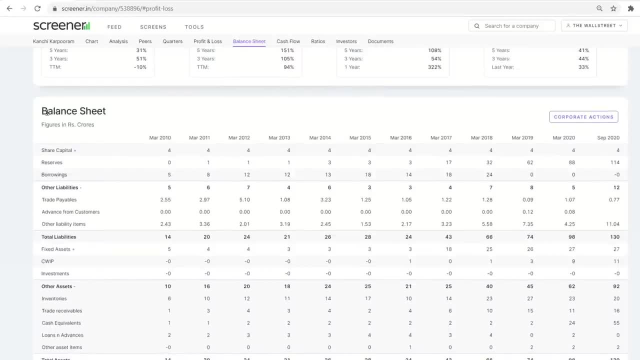 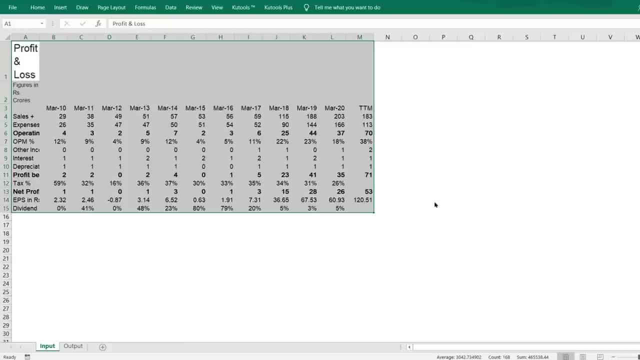 Once you click on those, you can create a copy of this also. So select the entire thing till here till total assets, control C and then control V. Simple right Copying balance sheet and profit and loss account from your website. 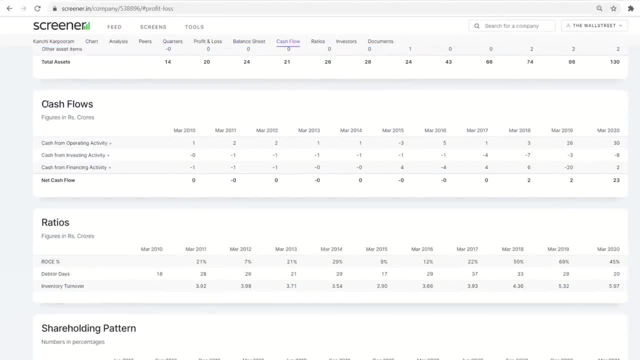 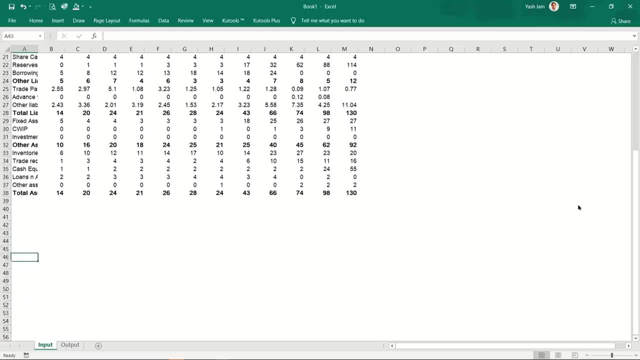 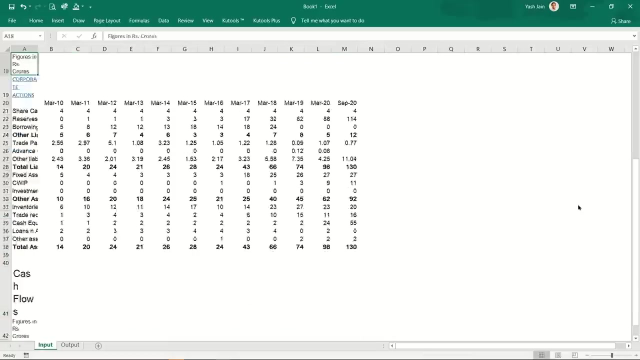 Okay, Going back to screener, simply will be selecting this cash flow statement that is just below the balance sheet. copy it and paste it here. Paste it here, Right. Simple, Very simple activities till now. Okay, Once I have this data, see it's, it's very difficult to process that. 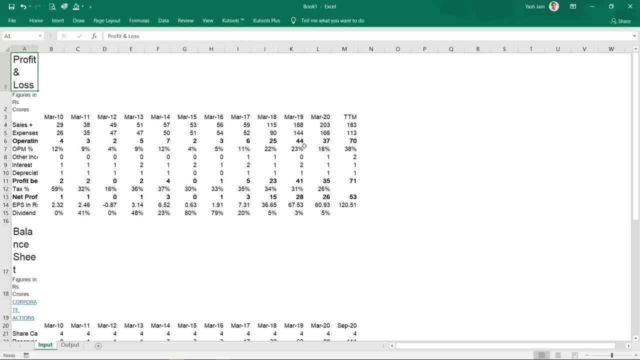 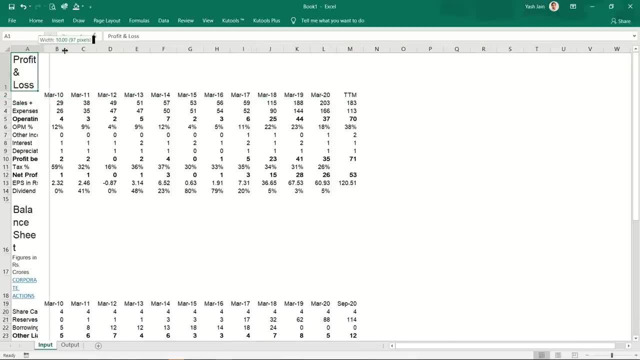 So I'll be just putting it in a proper format. You can follow up with me. So what I'll do is I'll just delete this. figures and corrodes. I know these figures are in corrodes. I'll expand this a column. 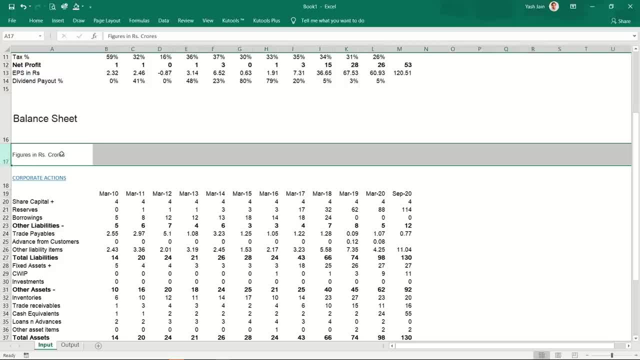 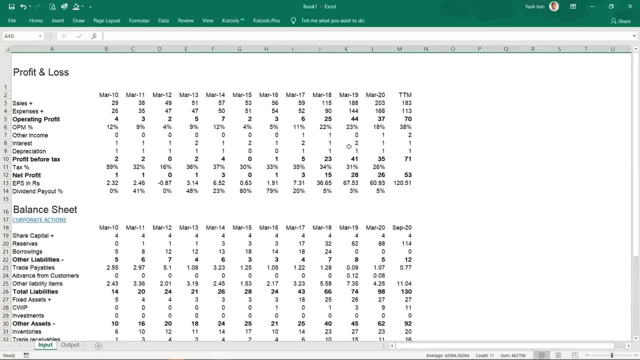 Right, Then I'll be deleting this figures in corrodes and I'll be deleting this figures in corrodes. Okay, This is my input data. I have not started to analyze here, but one thing that I see always while I am analyzing any company- and this is the single most important parameter, that is consistency. 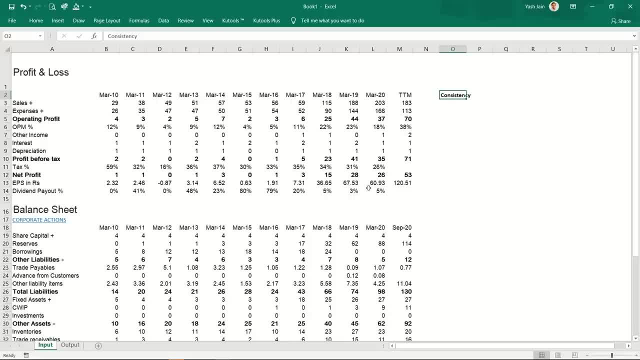 Consistency, Consistency, Consistency of sales, consistency of depreciation, consistency of your asset growth. I want the company in which I'm investing to be very consistent. I don't want except like exceptionally sharp rise in profits and next quarter or next year. 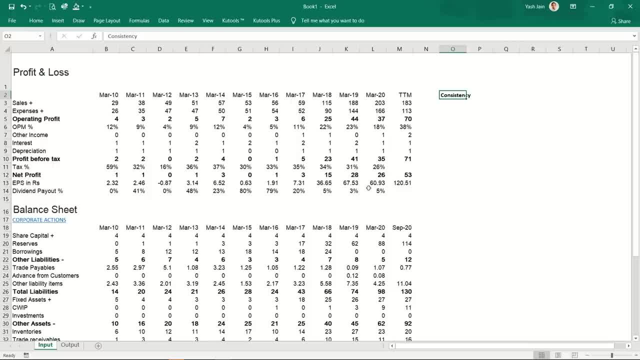 exceptionally sharp decline in profits. That's. that's not in my investment category, and retail investors are not able to time the markets, So you should. you should also not try to do that. Okay, The only thing that I'll be focusing on is consistency. 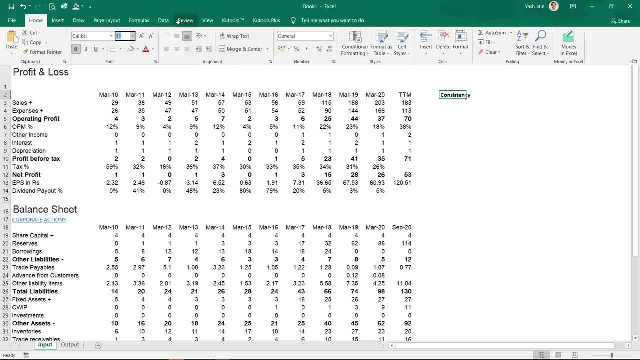 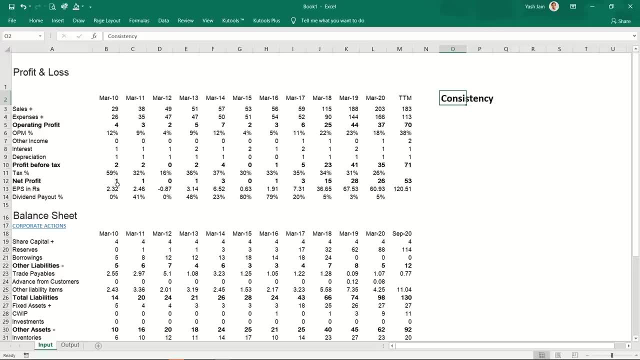 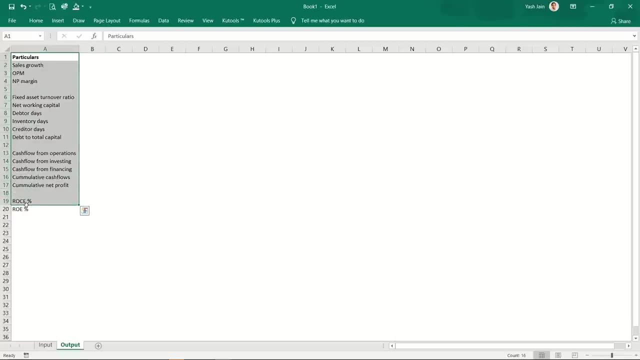 Let me like, Let me increase the font size here. Okay, Right, This is my input sheet. Whatever data I need for analysis is ready here. Then I'll go to my output sheet. I'll be calculating only few ratios here, few ratios here, and we'll be trying to interpret. 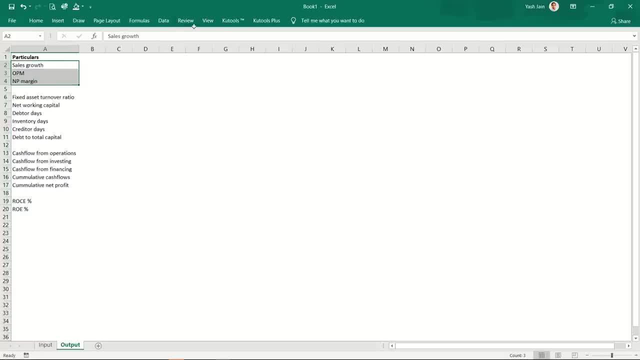 this, Okay. So first of all, these ratios that I'm highlighting now are related to your profit and loss account. But before doing that, first of all, let us get our years data here, Okay, This equals to: and I'll just link these years so that it becomes relatively easy to understand. 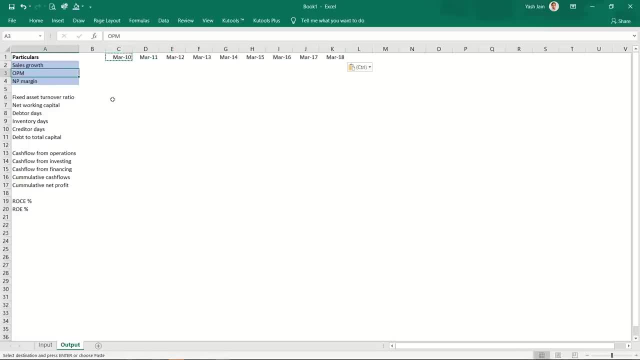 about which year I'm talking about. So first of all, I want to see the sales of the company in an upward trend. Sales should always increase because we are in a country that is inflationary in nature. We are in a developing economy. Inflation is very high in our country, Right? So even if they are not able to increase the volumes of their year, they are not going to increase the volumes of their units sold because of inflation. their sales are meant to be like higher, right. 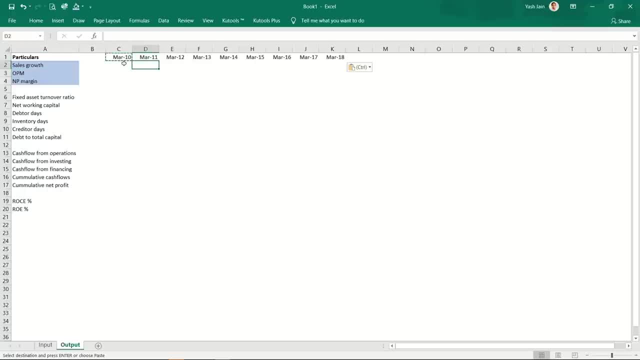 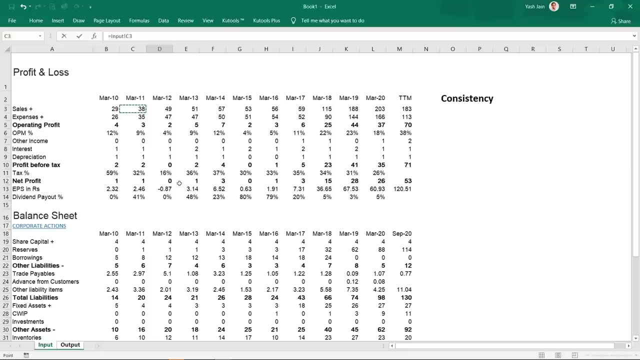 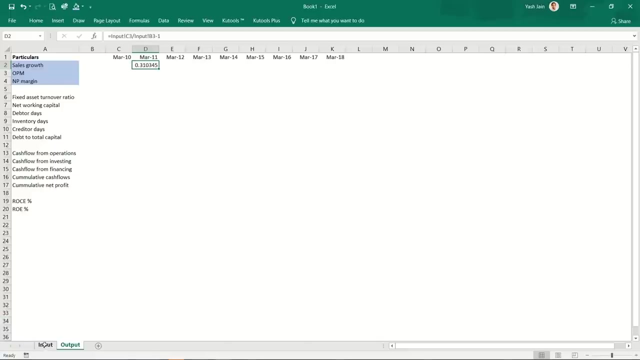 So I'll say I want to calculate growth. So in in in the column here, March 11,, I'll say: equals to last year car. or like this year car sales divided by last year car sales minus one. simple this simply telling me the. 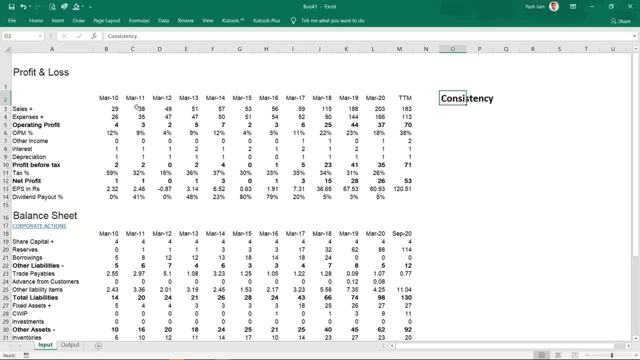 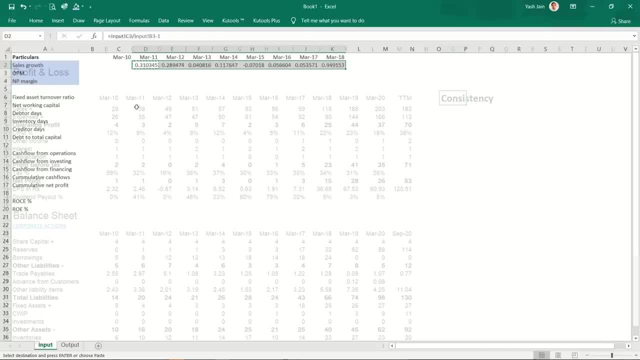 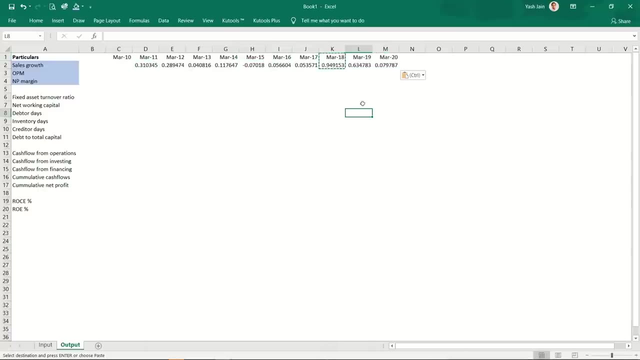 sales have grown from 29 to 38. That is Growth of almost 31%. I'll copy this and I'll paste it. Okay, Okay, I should have taken it till this, And I'll just convert them into percentages here. 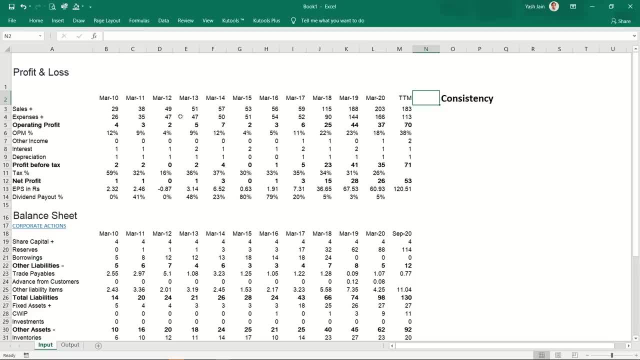 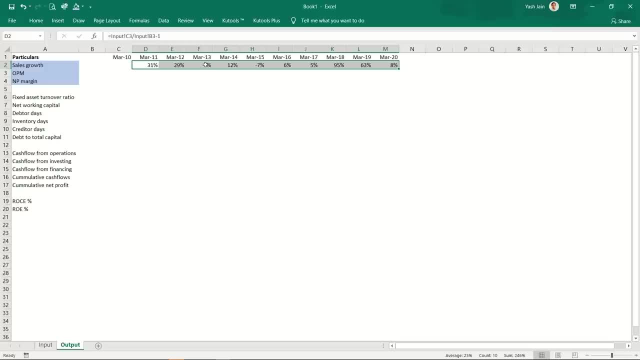 Now you can see, see it's. it's very difficult to analyze it this way, but now it becomes very clear. The sales have been growing very rapidly: 30%, 29%. Then there was a fall In 2013,. then again it rose to 12% and then there was a fall in 17.. 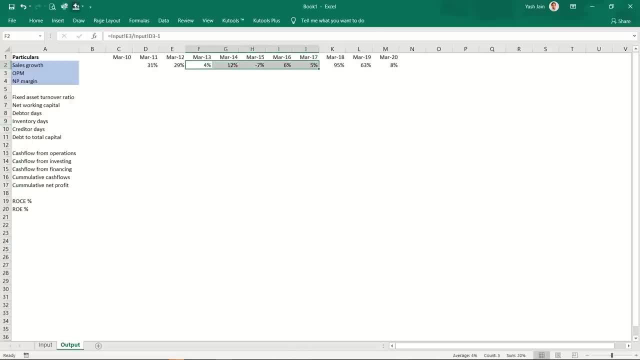 So I can clearly see I think during this period they were struggling a lot: 13,, 14,, 15,, 16,, 17 sale was like struggling, as in sale was not growing, It was only growing at the rate of inflation. six, five, six, 7%. 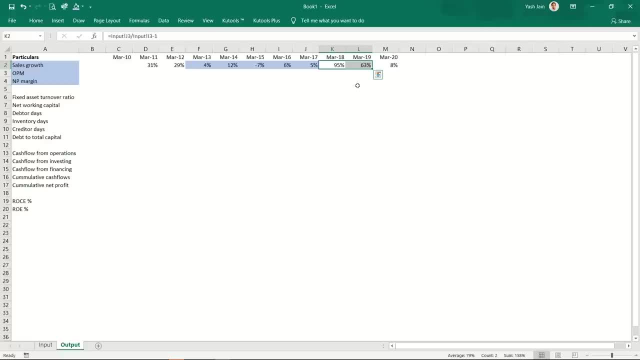 I'm not very happy about it. but look here: 95%, 63%. So it's a very, very good growing company, right, Though they are not that consistent. So they are not that consistent. So they are not that consistent. 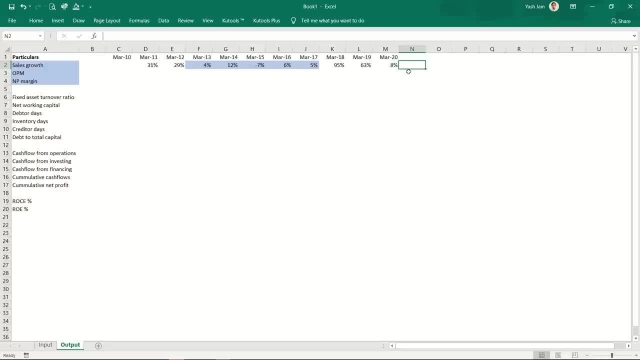 They are not that consistent with the growth, but still they are going very rapidly. If some year they are not able to grow, then in a couple of years they are able to catch up. So I'm not very satisfied with the consistency but I'm comfortable with till till some extent. 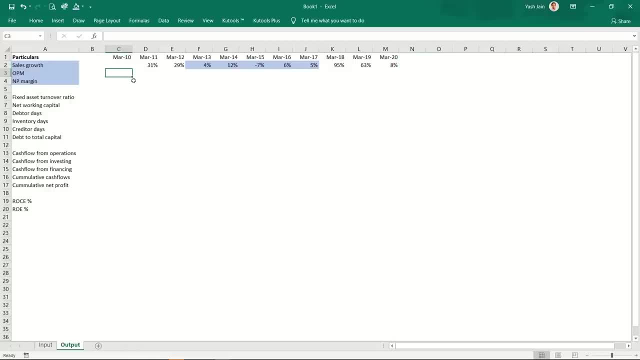 Okay, Then operating profit margins. These operating profit margin means how much profits you are able to generate before paying your interest and paying your taxation. This is basically your EBIT. Okay, Before paying your interest and taxation to government, how much profits the company are? 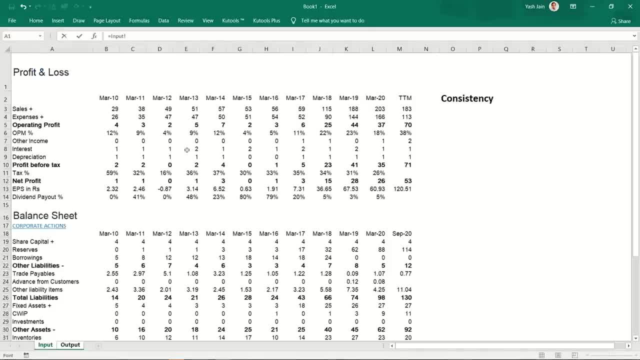 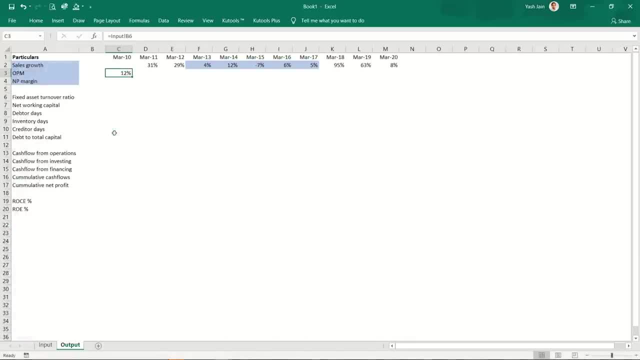 generating. So I'll say equals to, and I'll just link it here, This side. I've already calculated operating profit margins for me and I want profit margins to be increasing. right, I want my company to profit to be growing. So I'll say control C and control V. Okay, 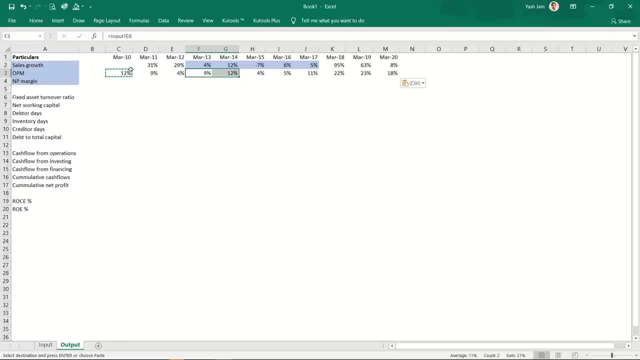 And you can continuously see in this, in this, like 12% to nine, then four, then nine, Okay, And you can continuously see in this, in this, like 12% to nine, then four, then nine, Okay, And you can continuously see in this, like 12% to nine, then 12.. 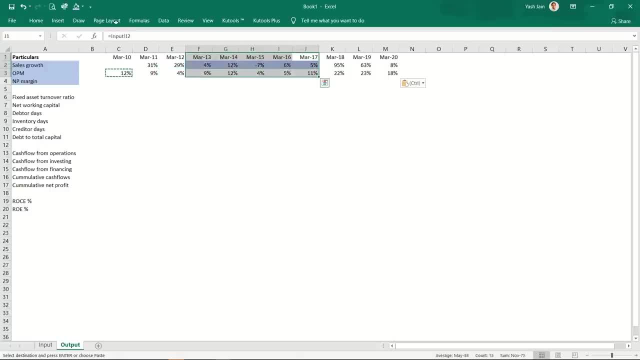 Okay, And you can continuously see in this like 12% to nine, then 12.. So after this, after this bad phase was over, I think they've done pretty well. They are continuously able to maintain 18% or more profit margins since last two, last. 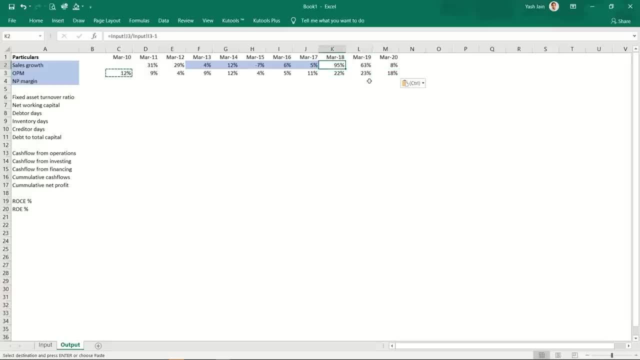 two to three years. this company is doing really good, a good sales growth: almost double sales in 17,, 18,. almost like 1.5 times or 50% growth in 19.. And because of like COVID situation, I can give them this benefit of doubt that their 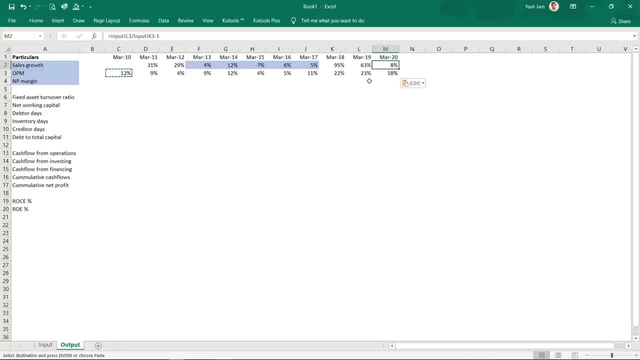 sales have only grown by 8%. Okay, So they are more than they had right. Others were like, like any, many companies were closing. People were not able to perform at all. Even if they are going 8% in tough times, I'm comfortable with it. 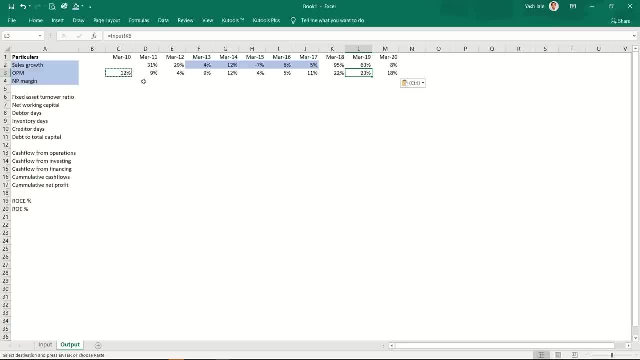 So gross profit margins was very hazy in last couple of years, But in last two to three years I think they've been consistent around 20% That's. that's a good sign for me that this company is entering into a phase where it 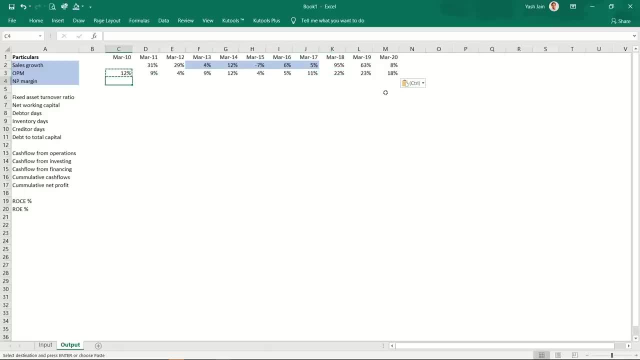 is becoming much more stable. Okay, Net profit margins. Net profits are what is finally left after paying interest, taxation, what is finally left with the company, So I'll say equals to net profit margin- is your net profit divided by sales. So net profit, this one divided by sales, and I want it in upward trend. 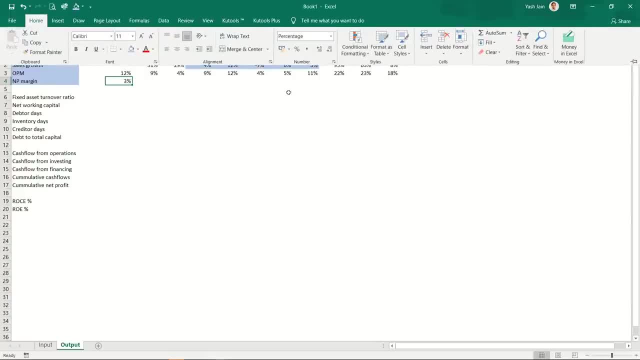 Let me convert this into percentage, So copy paste. okay, And now this makes me really happy. It was constantly stuck between 2%, 3% till here till here, But once they are out of this bad phase, they're really able to increase their operating profit. 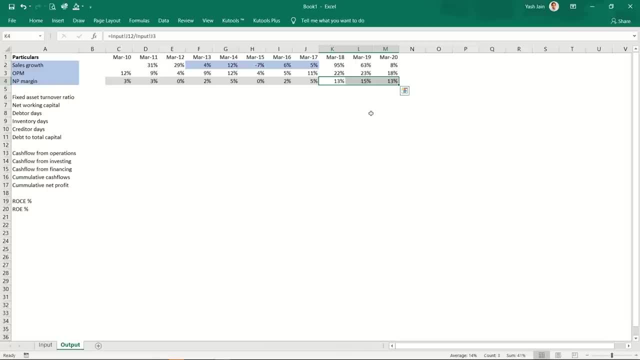 and that is getting impacted. that is impacting their net profit margins. So in last two to three years company have been really stable And 13%- 15% of their net profit margins have been stable. 13% net profit is healthy enough- not too good, but not too bad also. 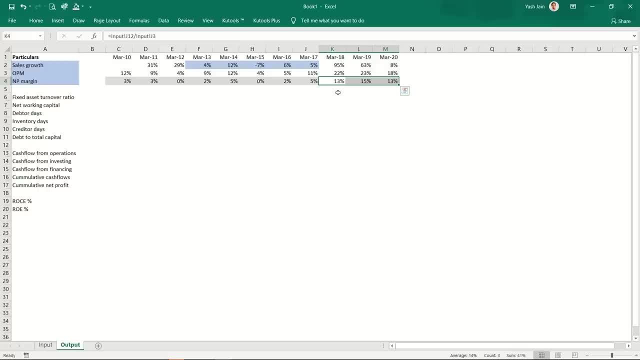 This is analysis of your profit and loss account. I'm not making it very complicated. Obviously, a lot more things could be done, but we learn them slowly and slowly. We are just starting, So this is good enough. Sales is growing and my operating profits are growing and my net profits are growing. 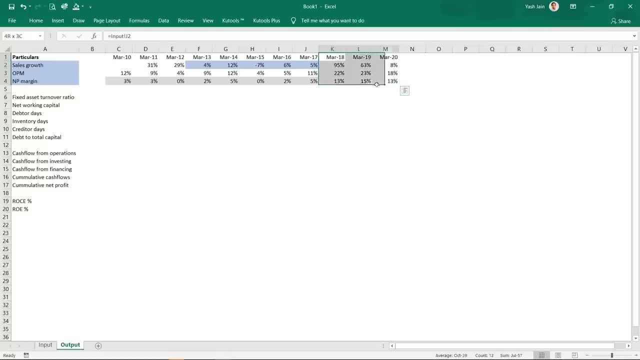 at a very consistent pace from last two to three years. This brings me some satisfaction that this company is improving with time. Okay, Then let's move towards balance sheet. These ratios are related to your balance sheet, right. First of all, fixed asset turnover ratio. 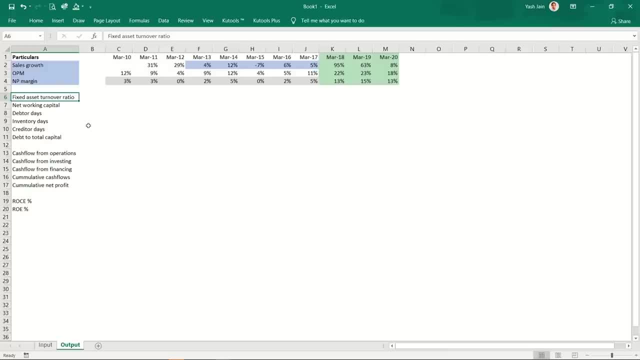 Firstly, let us understand what does this ratio does? What does the ratio tell us? Fixed asset turnover ratio means for every one rupee invested in your fixed assets, Remember, remember that business cycle: like you raise some capital, you purchase fixed assets from that and fixed assets were used to do your turnover. 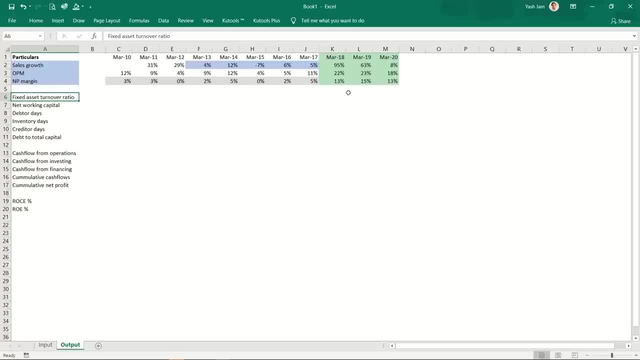 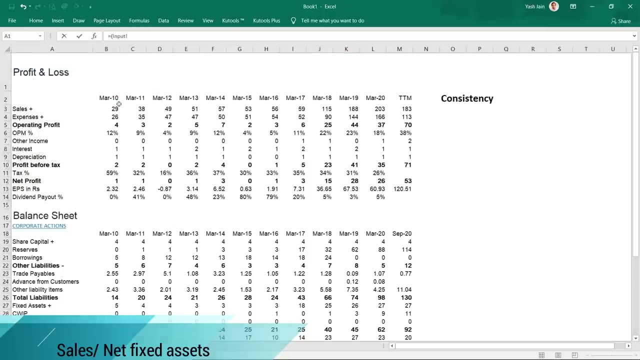 So fixed asset turnover ratio tells you how many times of sales you are able to generate by putting one rupee of capital in the business. So I'll say fixed asset turnover ratio is sales divided by your fixed assets. So sales divided by fixed assets. 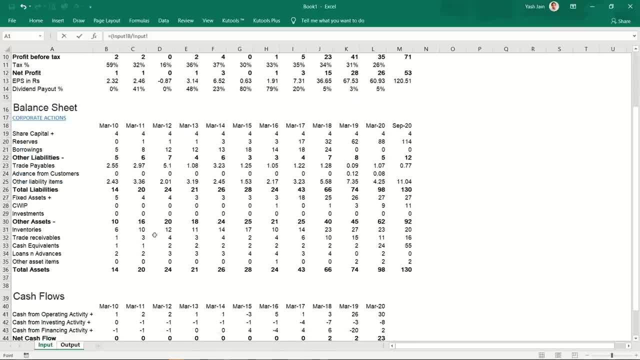 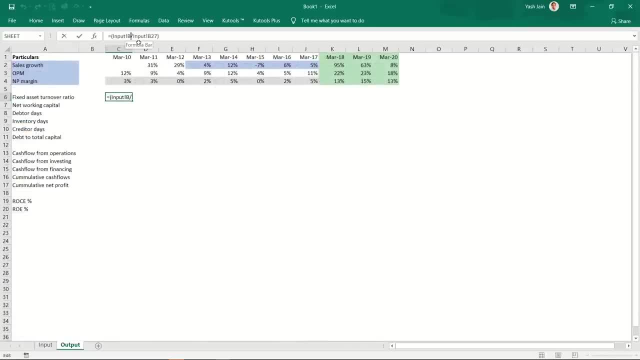 That is Okay. Okay, That's given over here. Okay, Enter. Oh, I think I've made some mistake. Sales divided by fixed assets: Copy Paste. I would want to see it in increasing trend. See what does this? 5.80 tells me that for every one rupee invested in the business, 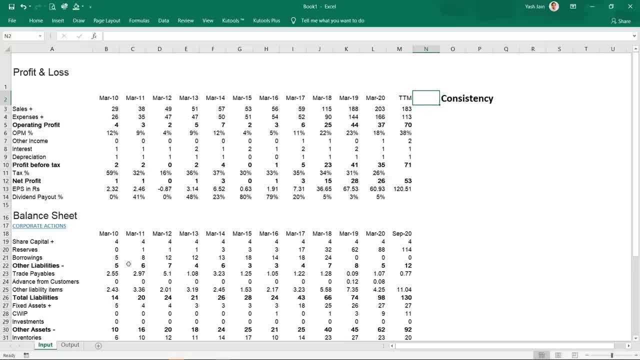 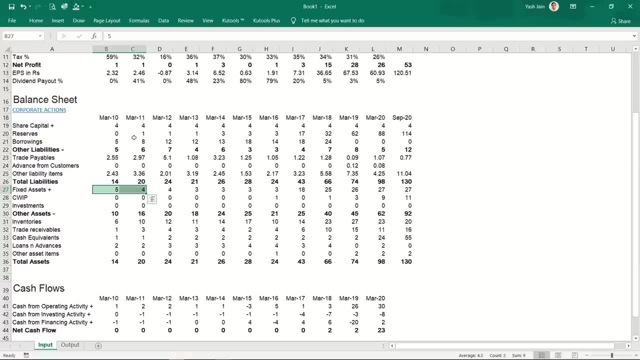 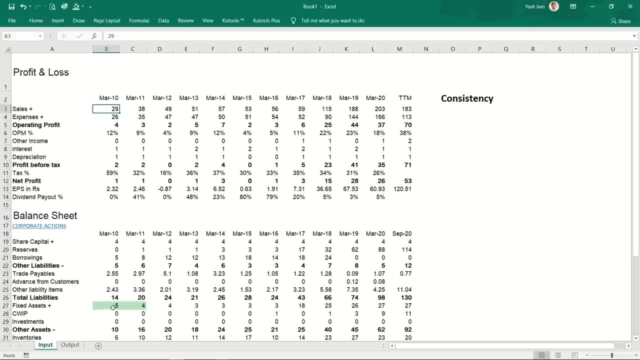 I'm able to generate six rupees sales. So their fixed assets were around here. Their fixed assets were around four crores, five crores And you can see their sales were around 20, 30 crores. So by putting five rupees they are generating 30 crore sales. 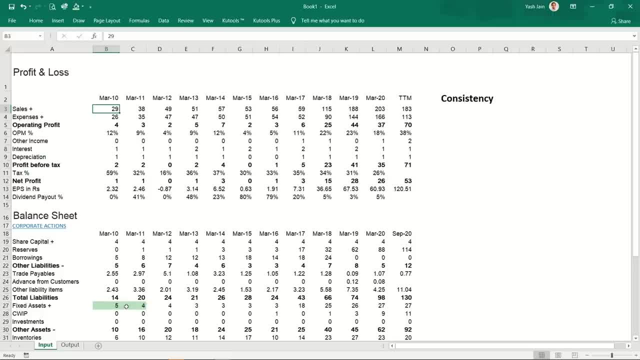 That is, by putting one rupee, they are generating almost six crore rupees sales. And till here, till 2017, like till 2016,, their fixed assets were slowly and slowly, slowly and slowly reducing Because of depreciation and their sales was increasing slowly and slowly, but not at a 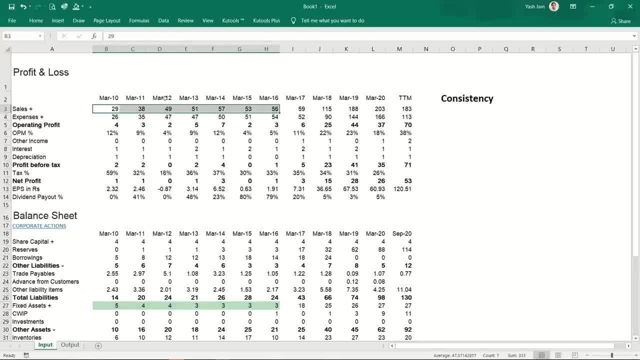 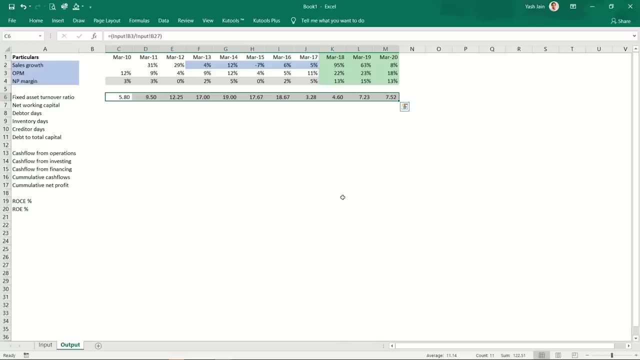 very rapid pace. Right Sales have even not doubled in these six, seven years. But once they started doing Capex, once they started purchasing new fixed assets, then you can see their sales skyrocketed. So that's a healthy sign for me that my company is able to generate maximum possible amount. 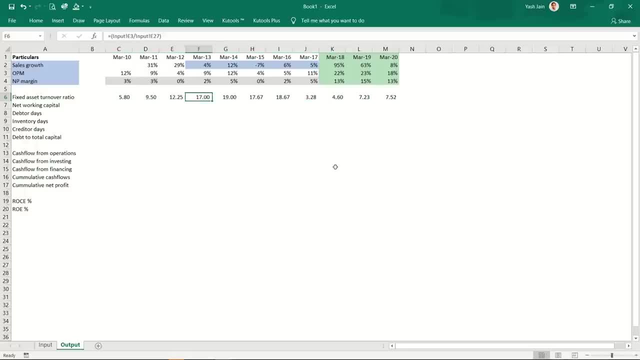 by investing one rupee in the business. So you can see here. It increased for a couple of years. Then it started going down, Then again like when this capital expenditure was done. so they've they've purchased plant worth rupees 18 crores. 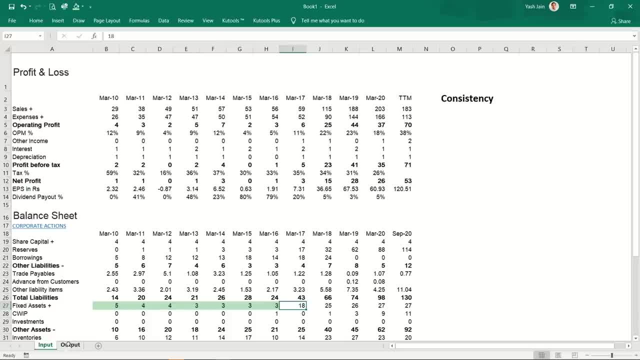 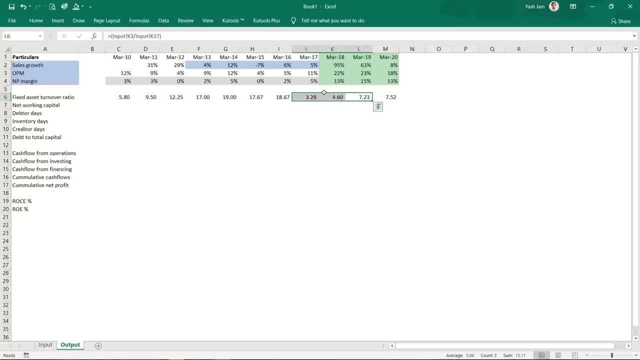 They cannot expand their sales in one year. it will take them a couple of years, So three to four to seven. this is pretty good, right? Their sales is continuously increasing because they've invested in fixed assets. From this point of time, I see that there is some consistency in them and that's good. 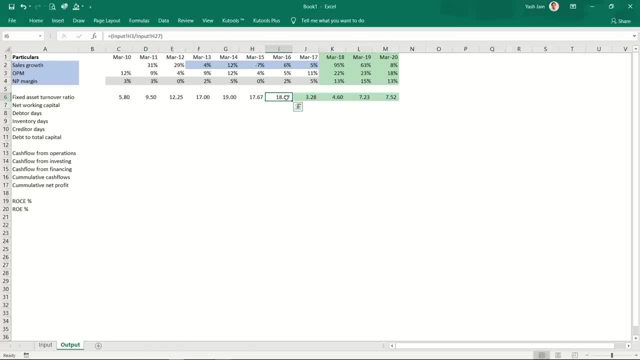 There is some consistency in them. They are also consistent here. Then they did a major Capex here, capital expenditure, that is, they purchased lots of fixed assets. Therefore, it went down and again started to increase. That's a healthy sign for me. 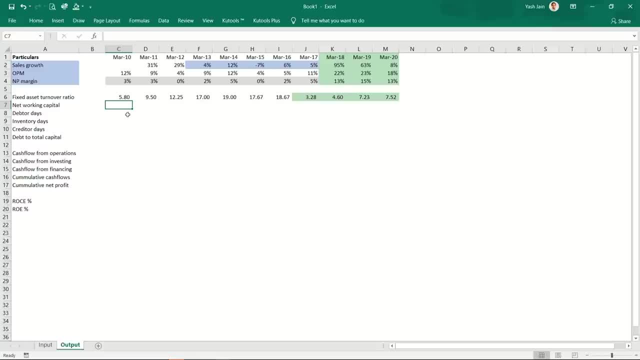 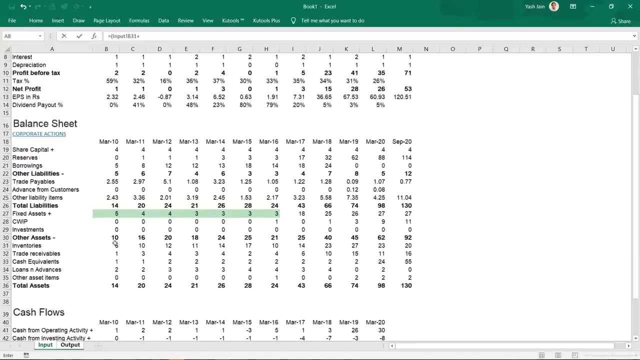 Okay, Then working capital, the lube of the business. So formula for working capital is debtors, like current assets, minus current liabilities, to simply put it. So I'll say: current assets- That is my inventory, Okay, Plus your trade receivables, plus your loans and advances, plus these other asset item. 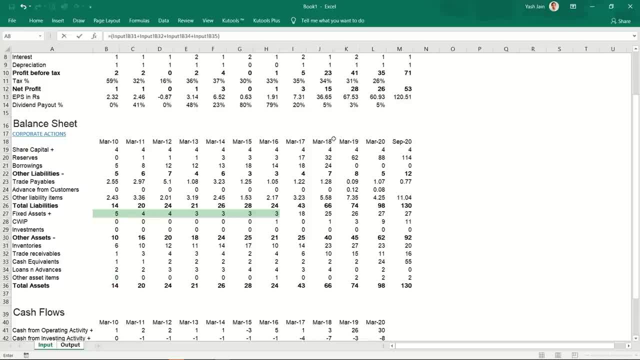 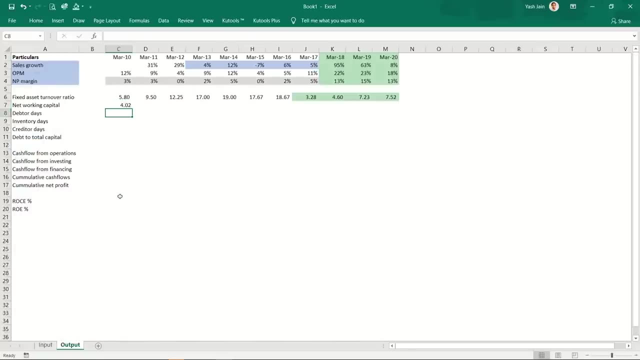 I'm not considering cash here. Okay, This is your total of current assets minus current liabilities, That is, your trade payables, then your advances from customers and then other liabilities. Okay, Enter. So working capital should be in sync with sales. 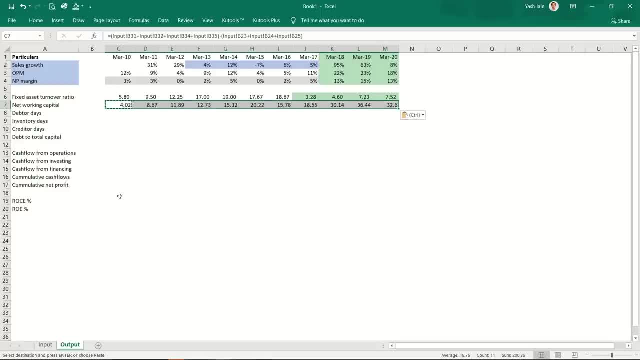 Okay, If their sales is increasing, they need to purchase more raw material and people will also be purchasing more from them on credit. They need more inventory to cope up with the sales, So it should be in line with the sales. Okay, You can calculate here a ratio called as net working capital by sales. that will show you. 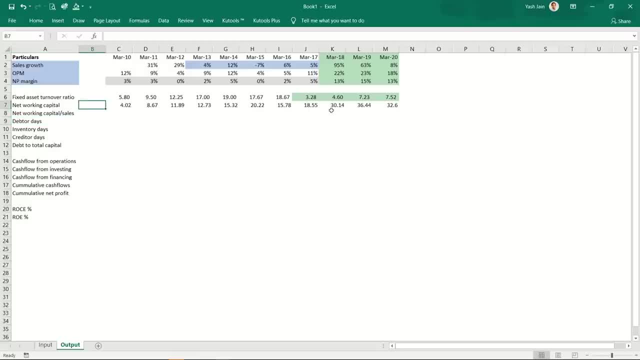 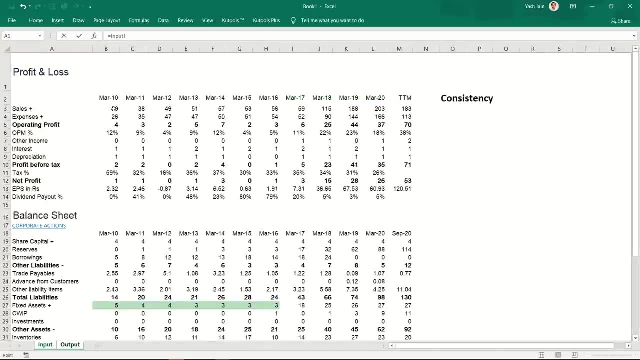 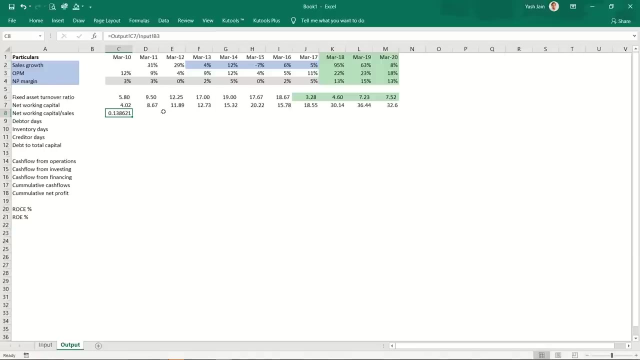 how much percentage of sales is captured by working capital. So it should be consistent enough, right? It should not be very consistent, It should not be very fluctuating. So working capital, this one networking capital by sales, Let me convert this into percentages. 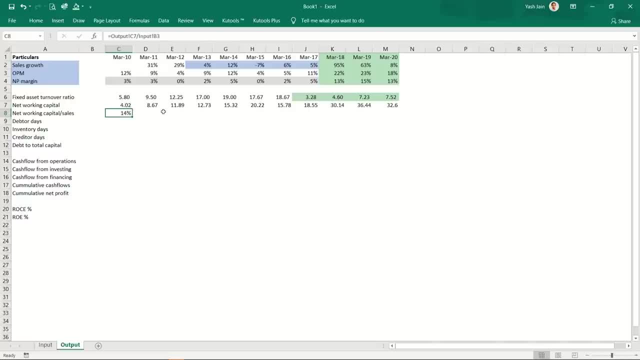 Okay, This means that working capital investment is around 14% of the sales. Let's copy and paste this. I want this to be very consistent. See, there was like working capital is around on an average 20, 25% of the sales in some. 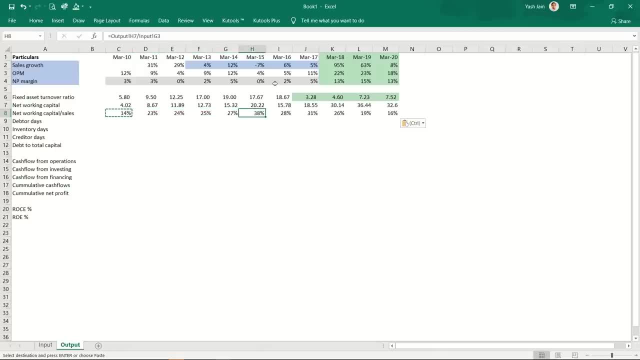 years It increased drastically When there was decline in sales but the working capital- there was lots of unsold inventory, Lots of people from whom I have to collect money. So it didn't decrease drastically but then it has been pretty consistent around 20, 25%. 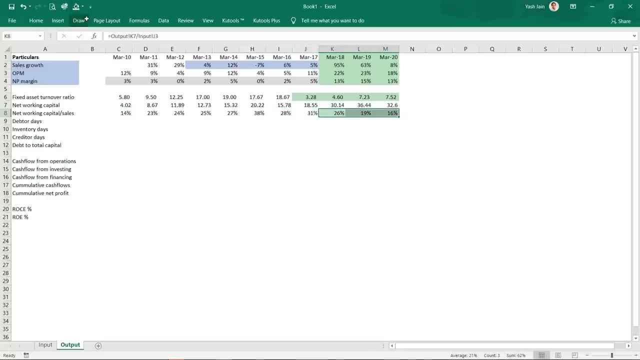 in last two to three years Right, And it is decreasing slowly And that's a good or positive sign for me. That is, my money is not getting blocked in working capital. Lots of people are not purchasing from me on credit. I'm not purchasing my raw material from people on credit. 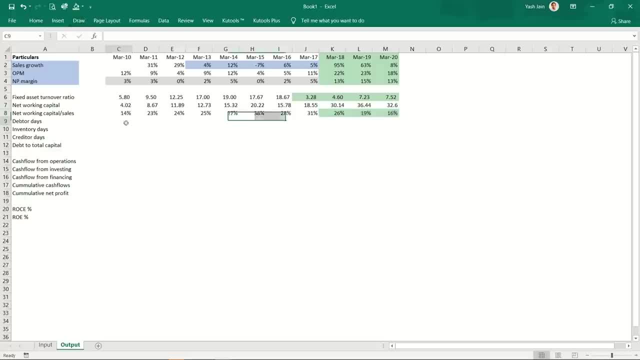 And I have sufficient inventory right. Okay, Then debtor days. This means the people to whom I am selling goods on credit and how many times they are paying me. So the formula is pretty straightforward: In a year, you have 365 days. 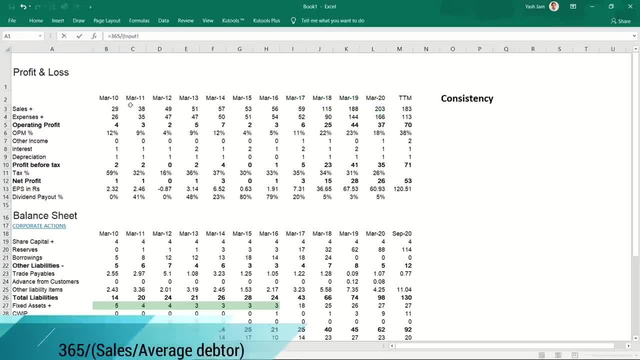 So 365 divided by sales, divided by average debtors- average debtors- debtors in this case- is returners Straight forward. Let's say that you're a debtor, So you know this is your income, right? So if you look at this table, so last year, this year, 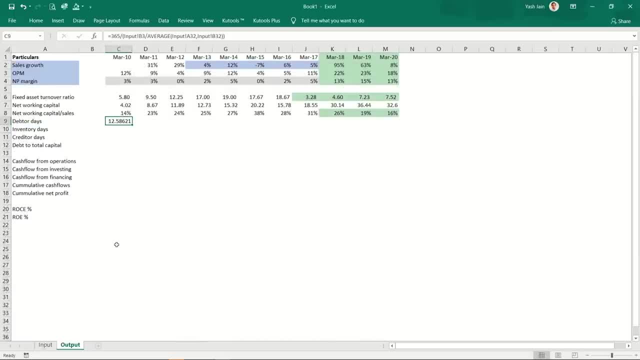 Okay, Let me convert this. Okay. So debtor days, that is, people are paying us in 12 days. It should ideally be consistent or should be decreasing. What's the meaning of this being increasing? That means to increase my sales. I am selling people on credit and in this environment it's very, very difficult to 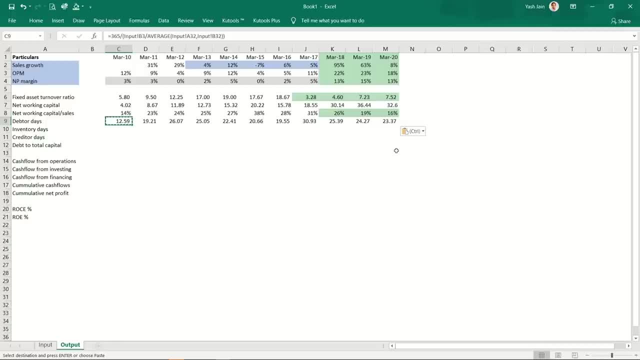 say that whether you will be getting your money on time or not. Okay, right, so it should ideally be decreasing or it should be very consistent. so last two to three years it looks pretty okay to me, 20 to 23 days and you can see here it was slowly increasing. 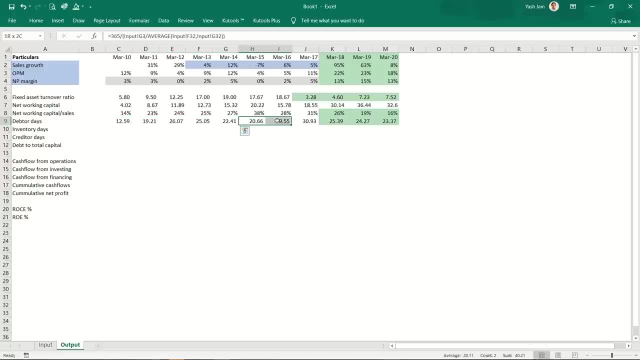 that's a sign of danger for me. but then again it started to decrease. then 17 may there was a sudden bump and then it normalizes around 25 days. that means the people to whom i am selling my goods starts paying me money approximately in 20-25 days. that is three to four weeks, that's, that's okay. 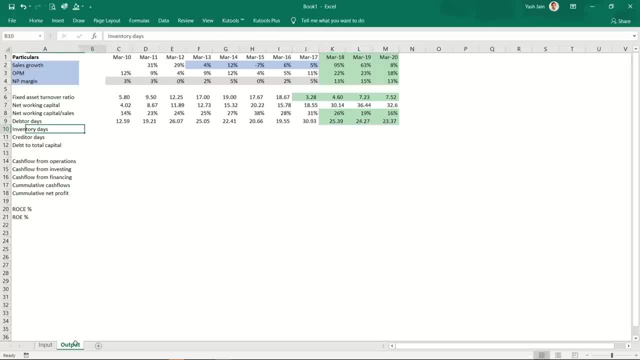 okay, okay. next is inventory days. that is for how much period i am holding my inventory, how much days it takes to me to get my raw material, convert it into finished goods and then sell it. so how much days it is taking. so the formula is pretty straightforward: 365 divided by 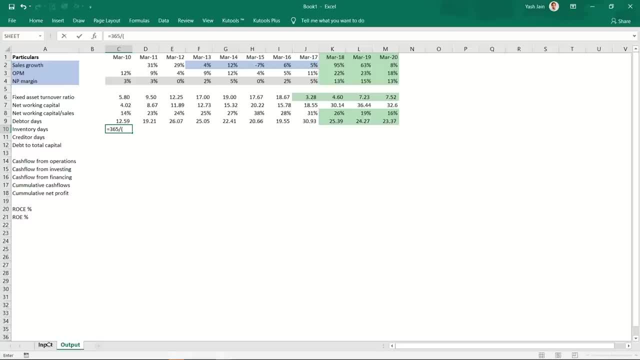 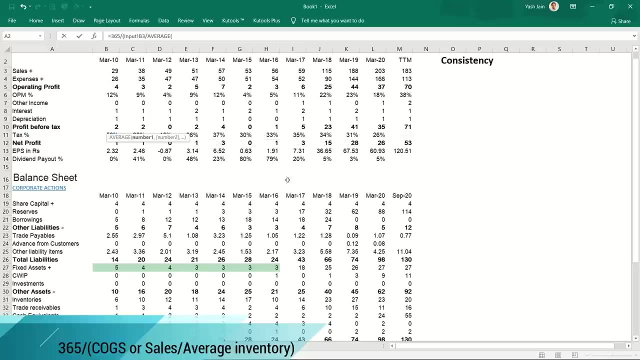 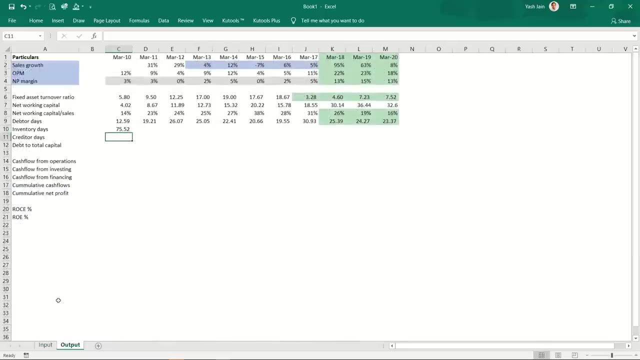 you average uh, cost of goods sold. since we don't have cost of goods sold here, we will be using sales divided by average inventory. that is, this and last year. okay, bracket close, bracket close and copy paste. okay. so what does this tell me? this tells me i am having like, like i'm having- inventory. 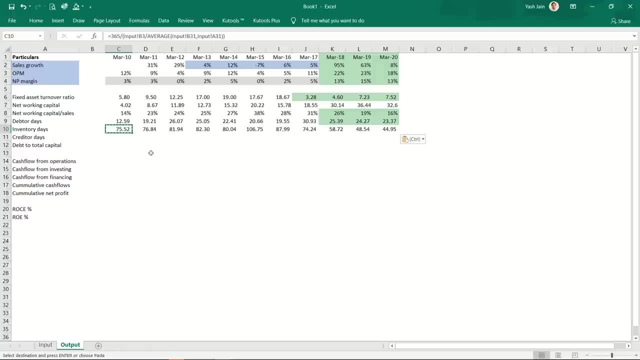 to mac, to, to, to, to match my next 75 days sales. it's too much of an inventory right. if you are a very good company, as soon as you purchase or as soon as you make some finished goods, it should be sold very immediately. so it should be in a decreasing trend, but it should not be very extremely low, right it? 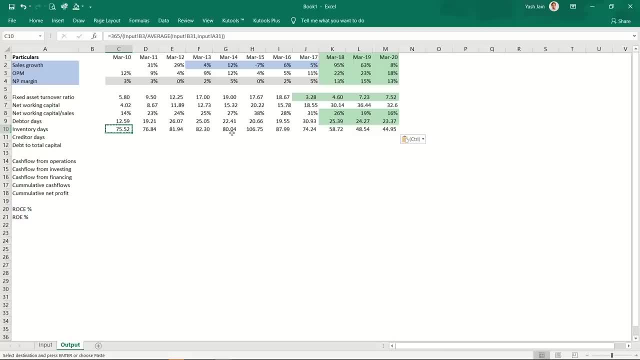 should be in a decreasing trend, but it should not be very, extremely low. so you can see here it was increasing. that was alarming for me why the company is able like, why the company is taking so much of inventory. that means it's not able to sell it right. its sales was not growing very fast, but it was like producing. 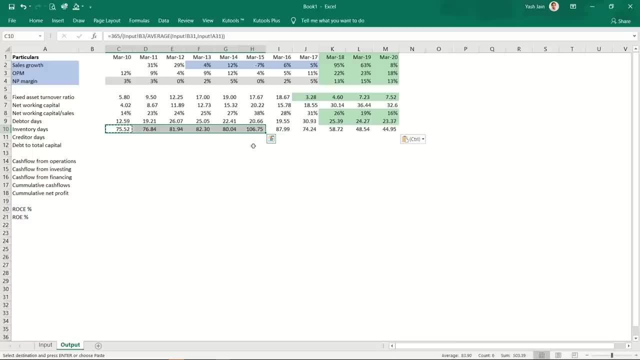 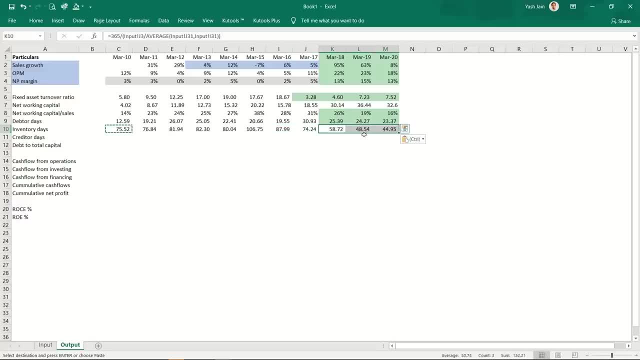 last four or five years and you can see consistently, they have been able to reduce inventory days at a very normal rate. it was increasing about two to three timesikle per month, which is to say five Sé low place. that's, that's healthy. okay, then creditor days means? and how many? 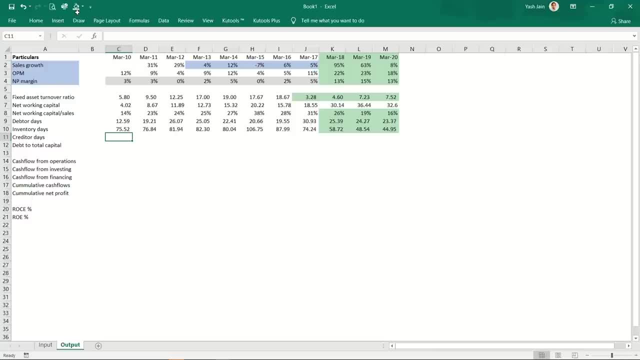 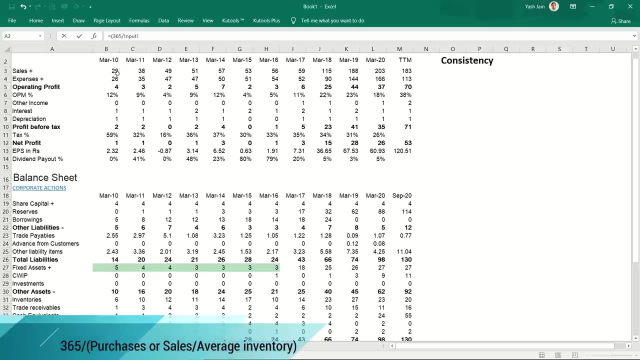 days, I am paying the person from whom I purchased my raw material. so the formula is pretty straightforward: equals to 365 divided by. I should actually be using purchases here, but since, since we don't have it here, I'll be saying equals to sales divided by average trade payables for this year and last year: average enter. 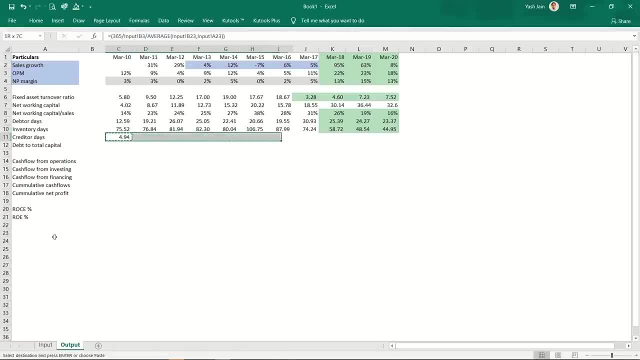 okay, copy paste. okay, that shows me. I am paying my creditors in a matter of two days, three days, five days. it should ideally be increasing slowly, and slowly, that is. I should be in a position to tell my creditors: if you're doing business with me, you have to do it on my terms. I'll be paying. 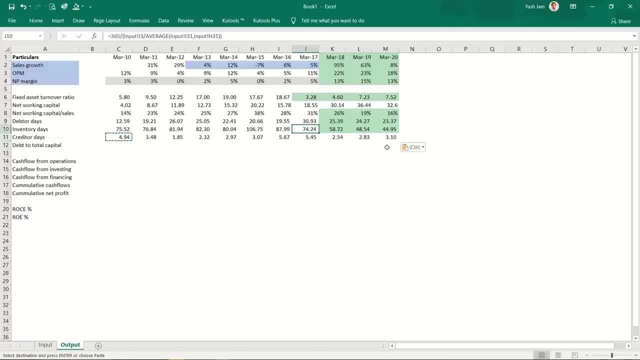 you in two weeks, three weeks, ten weeks down the line and my inventory days and later days should be decreasing because I want my money to be realized quickly from other people. so if I am purchasing on credit I should be paying them at a later stage. maybe it went two months, three months down the line and if 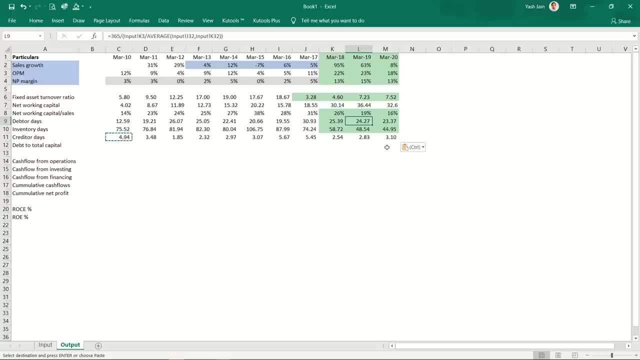 someone is purchasing from me, he should be paying me very immediately, maybe cash payments, or maybe in a week or two weeks. that would be the best situation. that would be the best situation, but I think the company is not able to do that like this is something okay for. 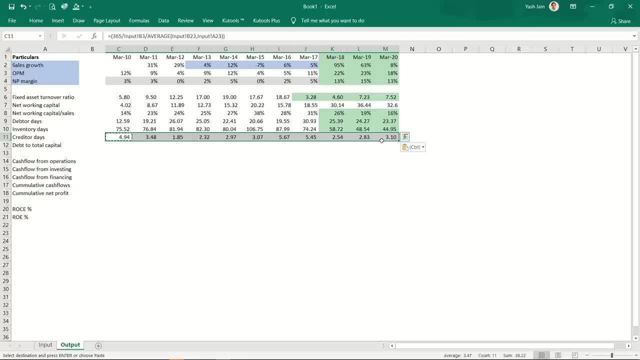 me since it has been like very constant throughout last ten years. but I would want the company to be in such position that it is able to negotiate the credit terms. if someone wants to do business with this with this company, they should be like they should be allowing a longer period credit. that's not happening with 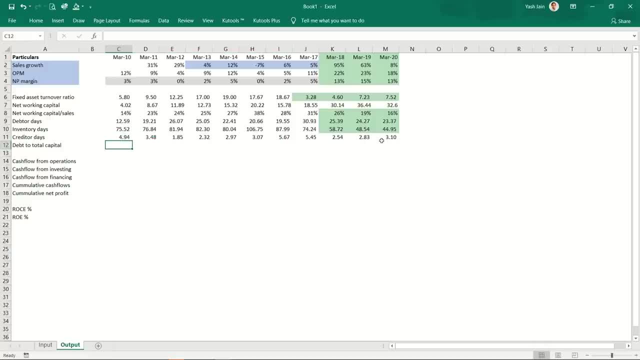 the company. and the last thing, debt to total capital. so we discuss this in the business cycle: to start the business, you need some capital and then ultimately, that business will generate profits and that will be used to pay off your debt holders and your equity holders. so if a 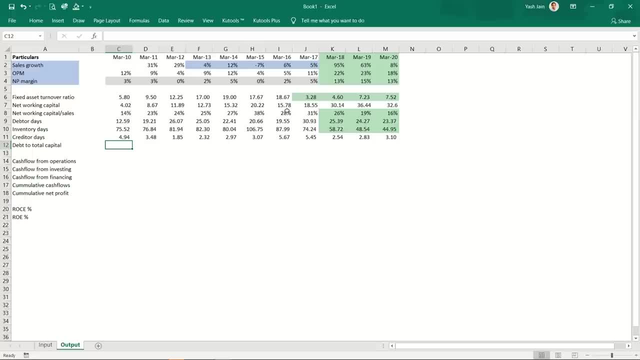 business is having lots of debt, majority of the profits that it is earning will be paid to debt holders in the form of interest. nothing will be left for you as a equity holder right and if this increases beyond a particular level and for one quarter. if the company is not able to do that, good. 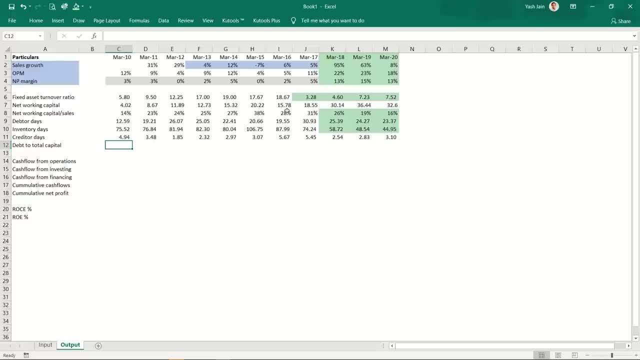 then what will happen? you will have to go for bankruptcy because you don't have any money and you have to pay some person. that person will drag you to the court and will file for bankruptcy. you don't want that to be happening to your companies, so always invest in those companies that are debt-free or at the 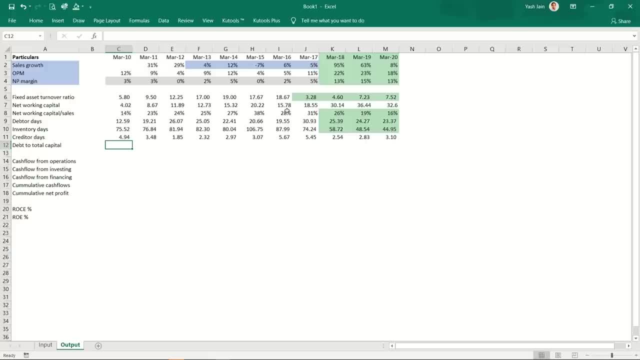 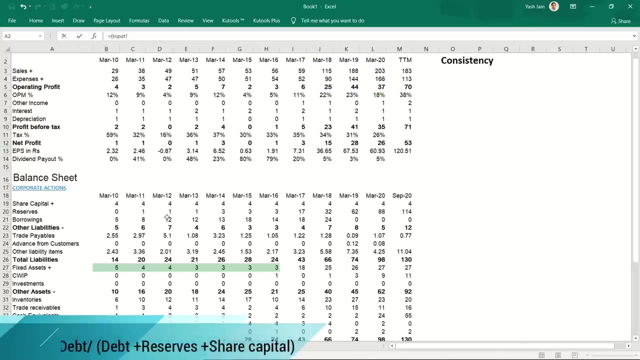 most. this is my typical defined line, at the most, 15% of debt in their capital. it's not written anywhere but to my personal experience, 10, 12, 15 percent tickets okay, but beyond 15, 18 percent, I think it becomes very dangerous. so equals to debt, to total capital. so debt is your borrowings divided by total. 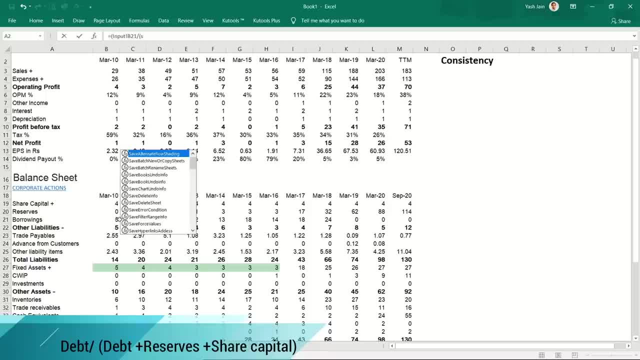 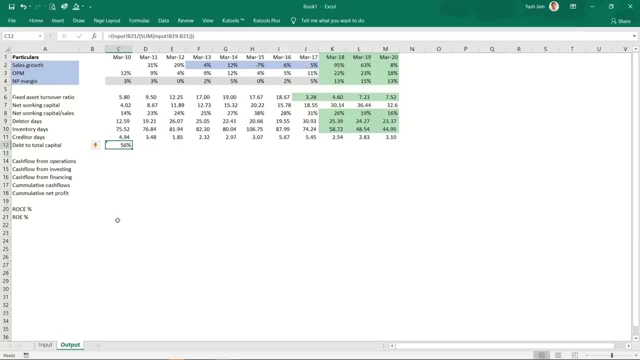 capital, that is your equity plus debt combined. so I'll say sum of share capital, reserves, borrowings, these things bracket loads so you can see this should be zero or this should be in a decreasing trend. so earlier, when they started in 2010, almost like one half of the capital was 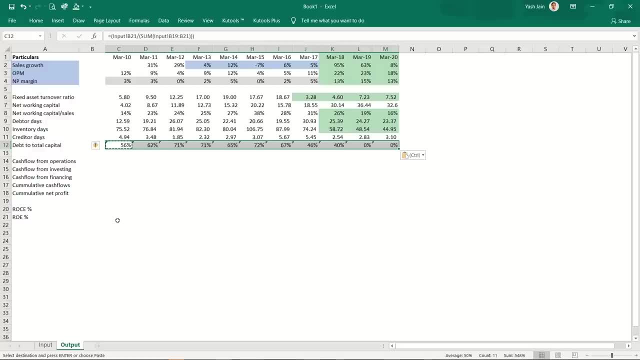 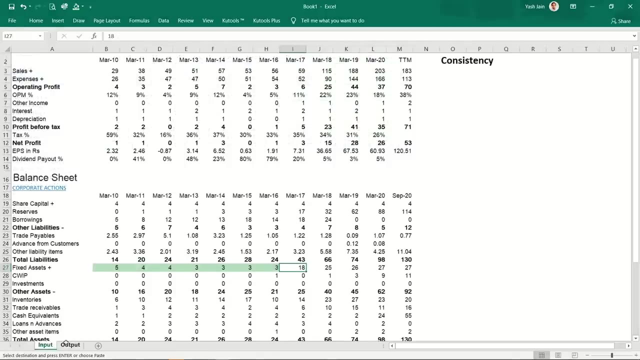 borrowed. then let's see what happened later years. then it was very consistent till here, and then you can see they have paid off all the debt as an investor. what a sigh of relief for me, like my company. imagine you don't have to pay any loan to anyone. you don't have to pay back any money to anyone. how relieved. 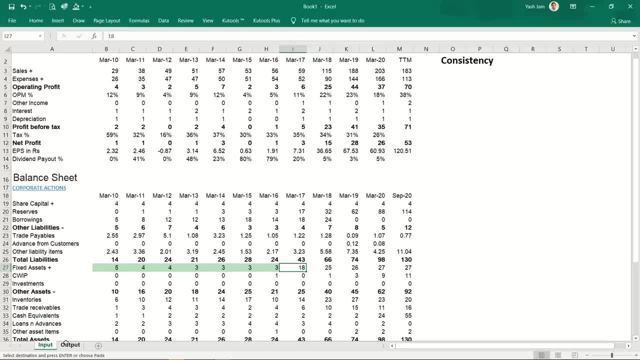 you could be. you don't have any external liabilities. you can utilize your funds and for the purpose of growth. so you can see company have paid out all its debt and that's a fairly good sign for me how it was able to do that? because it was. 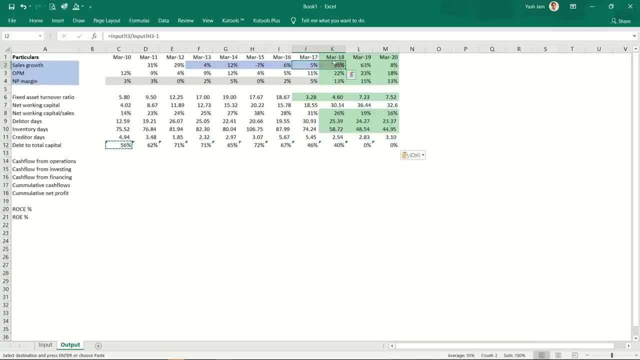 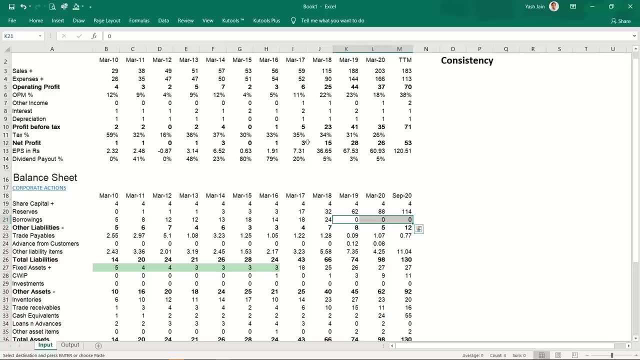 able to generate very quick sales. in this 2018 they was able to generate very higher amount of sales and their profits also increased. so you can see from 3 crores their profit increased to 15 crores and 28 crores and their total. 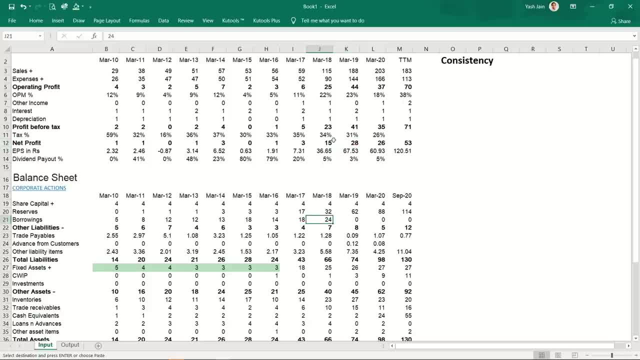 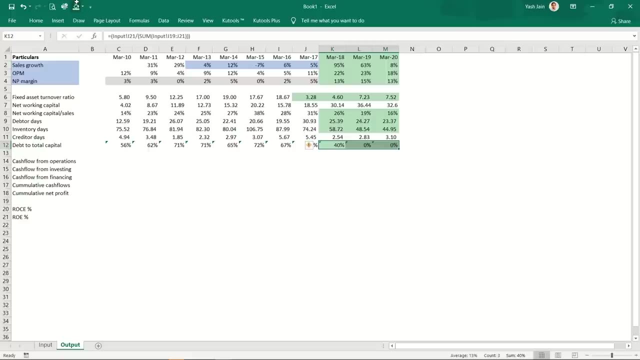 debt was hardly around 24- 18 crores. so, whatever they want, in two to three years they accumulated it, they paid it off and then now they are a debt-free company. what a sigh of relief. okay, this was balance sheet analysis, this entire thing. right, so I am pretty positive about the balance sheet analysis of this. 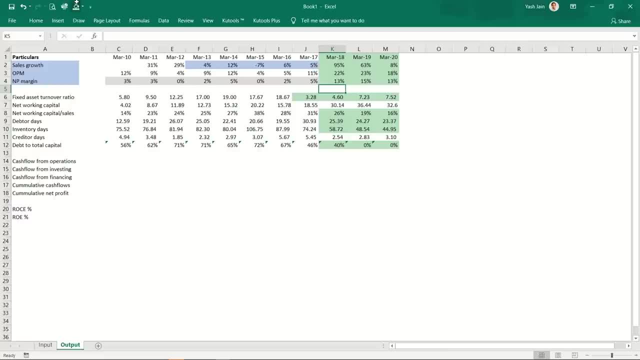 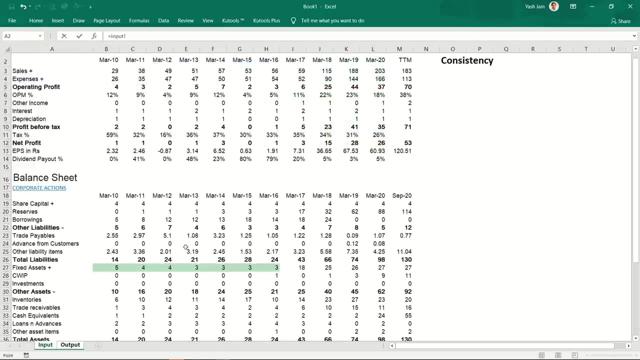 company. few ratios are not in its favor, but it slowly and slowly it's trying to improve. on some grounds it's. it's a sign of healthy and improving company. then what about this cash flow analysis? so let's get our data here. cash flow from operations, mmm, here cash flow from operations, then cash flow from investing. 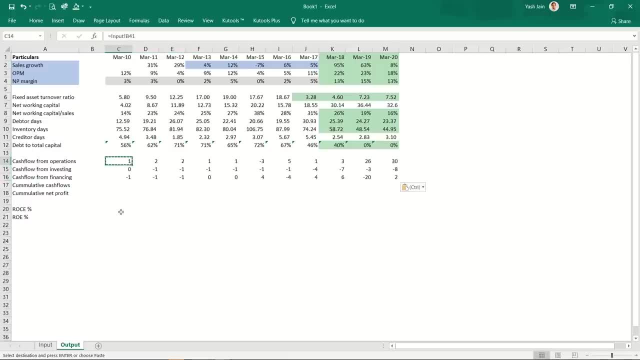 and cash flow from financing. okay, so I always want my cash flow from operations to be increasing. see, cash flow from operation means whatever. like the core business activity that you are doing, like in this case, Kachi Karpuram, is a manufacturers of like camphor and allied products, so using that, they are. 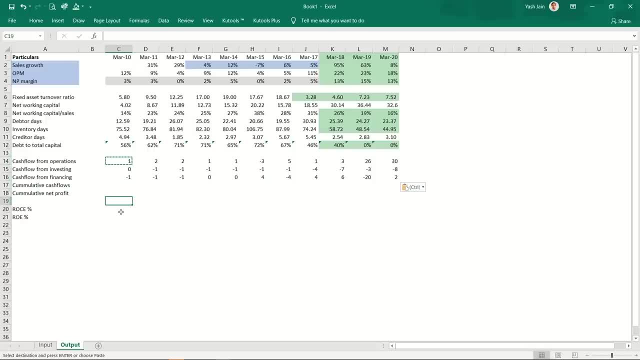 able to generate a lot of cash flow from operations, and cash flow from operations will generate cash, and you can see a good consistency here, like: if I compare this: let me insert one more row and let me get my net profits here, your net profits and cash flow from operations- if they are in sync, that's, that's the best. 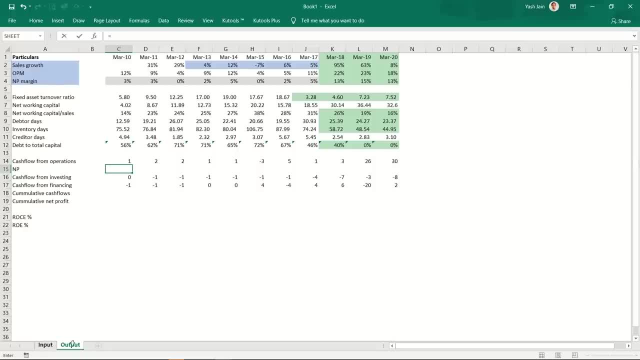 you can ask for, because whatever profits you are earning, that means those are cash profits, right, that means you can realize that profits very immediately. so you can see here most of the profits earned by the company: cash out of this 26 crore, 30 crores, the cash out of 28 crores, 26 crores, the cash out of 15 crore. 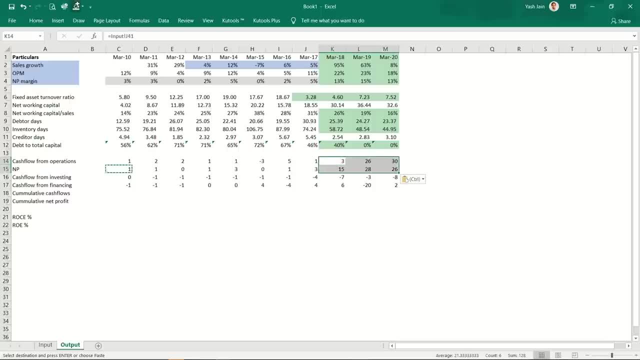 3 crores the cash. so slowly and slowly they are able to realize their profits in cash. see, profit is an accounting number. you can manipulate it very easily. if you go to a chartered accountant and like, if he wants to manipulate balance sheet, profit and loss account, it's not a very big deal. 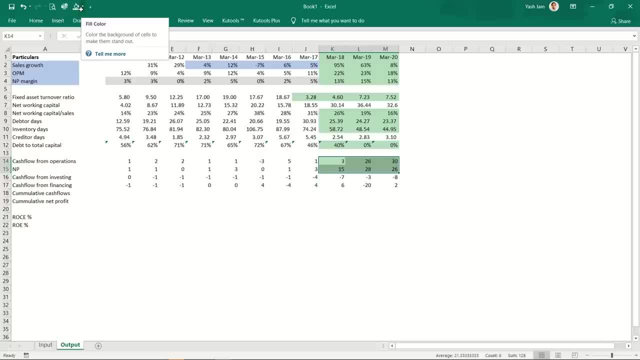 for him it's not a very big deal. this could be done very easily, right? but this cash flow statement is very difficult to manipulate- like manipulate, though, this can also be done, but it's relatively difficult. so this shows me a good consistency, like, whatever profits i'm earning, it is in the 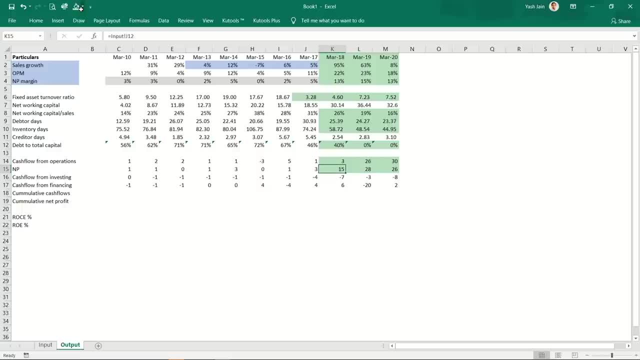 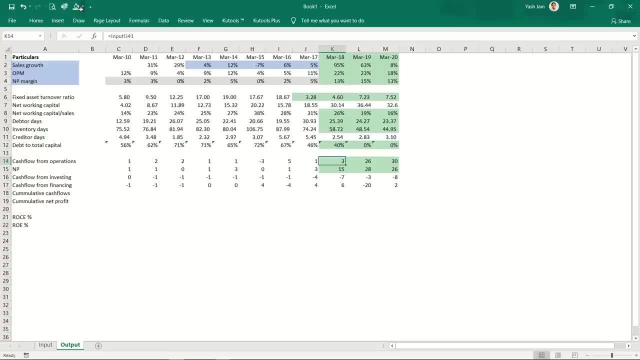 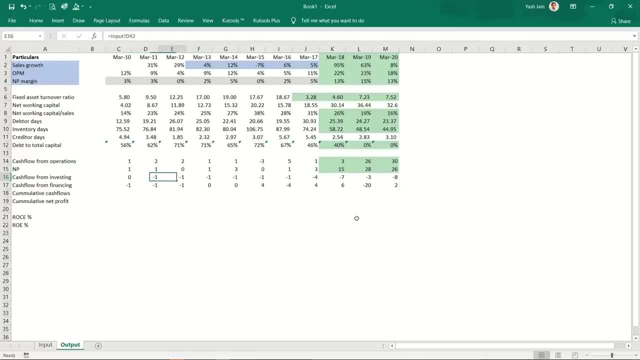 be negative, so understand this. this means this means negative means i'm continuously investing in my business in the form of fixed assets, that is, i'm increasing my fixed asset capacity. that will be helping me to generate more sales in future, then more profits in future, then more profits will lead to more cash availability. more cash availability will lead to more. 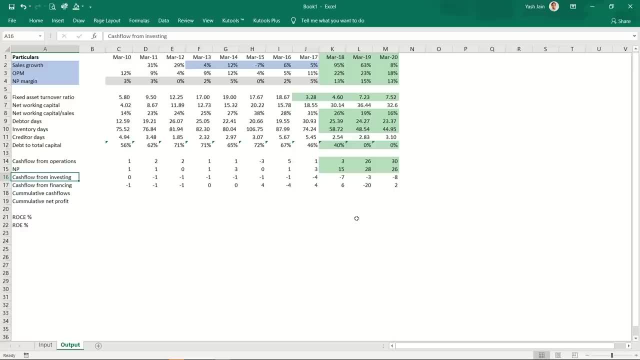 fixed asset purchases. that's a loop that is created right. so i want my fixed assets to be increasing. i don't want them to be increasing in a sudden way, but slowly and slowly, gradually. i want my investing activities always be negative. suppose my investing activities are positive. that means i'm 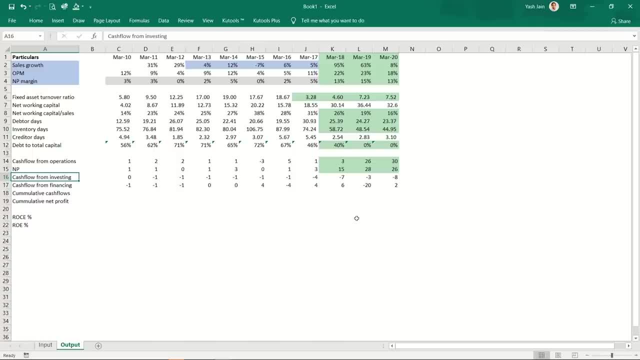 realizing cash from my fixed assets. that means i'm selling my fixed assets. i can do it once, twice, thrice, but maybe after two weeks i'm going to be using my fixed assets again and i can do it once twice thrice, three, four years. i won't be having any fixed asset. then what will i produce? how will i produce and? 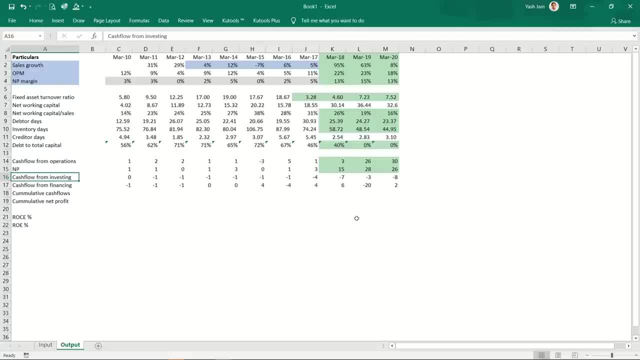 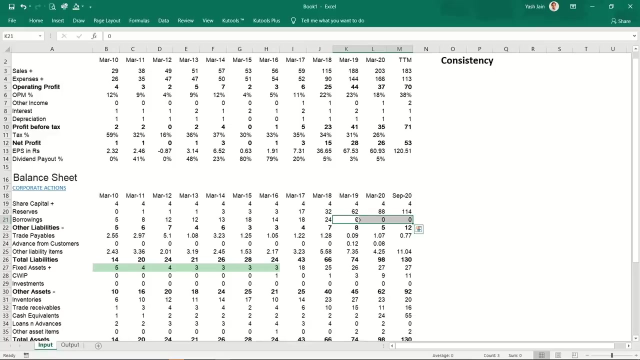 how will i sell if no sales, no profit. business is completely wrapped up. so you want these investing activities always to be negative. operating activity is positive. investing activity is negative. financing activity is also negative. see, these financing activities tells us that we are able to repay our dividend and our debt on time. the company, in 2019, paid all of its debt. 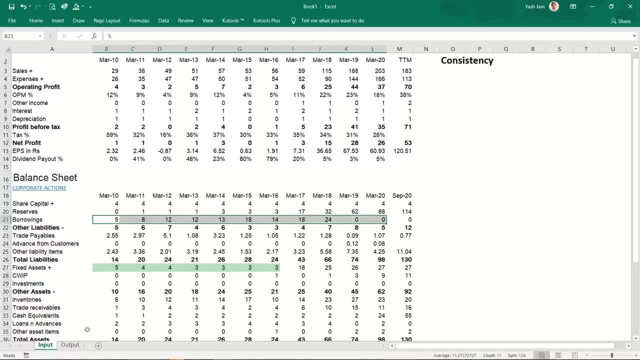 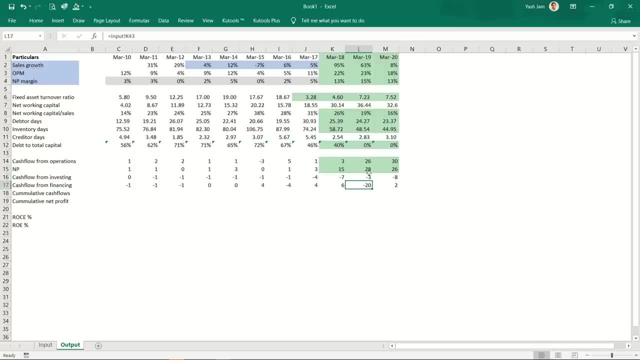 paid all of its borrowings here. so you can see it is negative 20 for 2019. that means the company is able to earn profits from here. invest some of the profits in your business in the form of fixed assets and whatever surplus has left it, it's paying back it, paying back its loan. 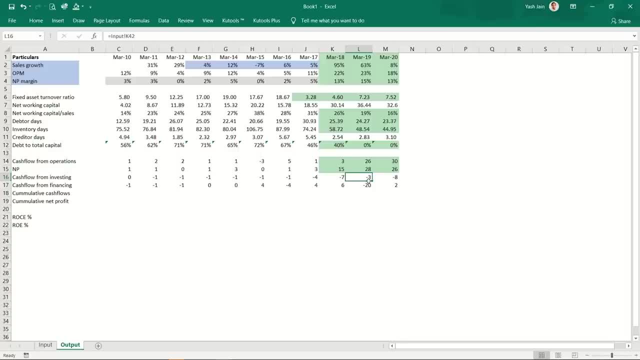 that means the company is able to pay back its loan. and the company is able to pay back its loan, That's a very, very positive sign for me. It is in line with your corporate finance principles. That's great. that's great. Then, one more metric that I use is cumulative cash flows. 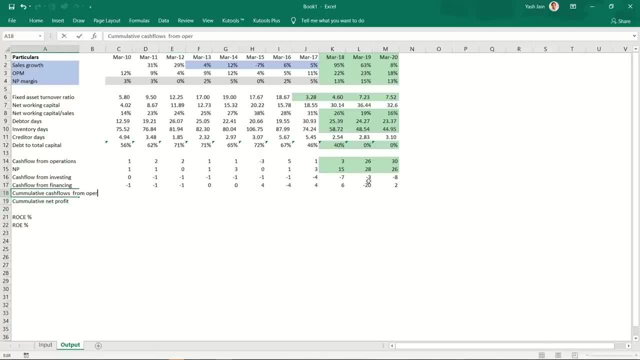 This is cumulative cash flows from operations and cumulative net profit. So this will be cash flow from operations this year, plus whatever I have earned till now. enter, I'll copy this and I'll paste it. okay, I'll do the same exercise with net profits. 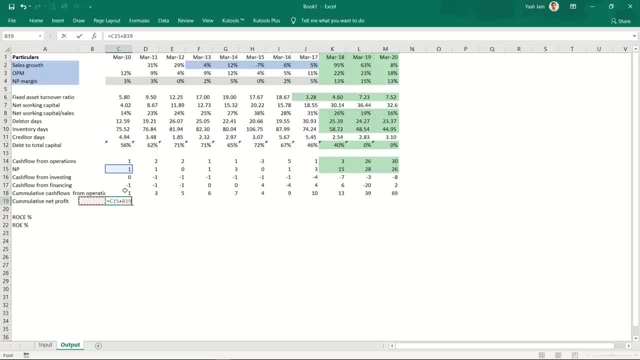 So net profits that I have earned this year plus my net profits of last year till now copy paste. So total profits realized till now are 79 crore and out of that 69 crore rupees have been realized right. So only 10 crore rupees is non-cash profits. 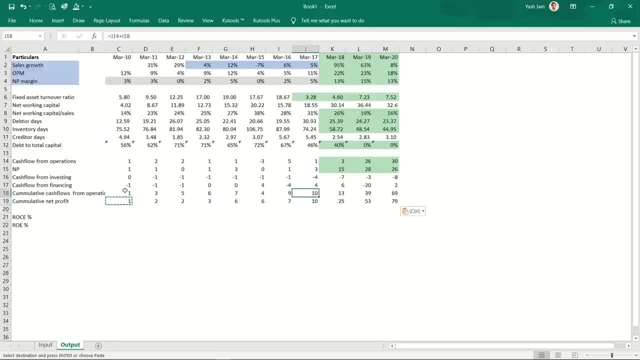 So you can see, maybe till here condition was 10 crores, 10 crores. Then my profits increased drastically but I have not received any cash flow for it. But now that is changing and, like in last two years, I think it have balanced out pretty well. 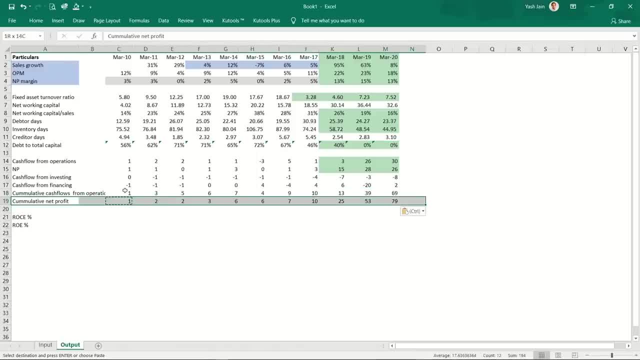 So this is my cash flow analysis, this complete thing. Okay. The other ratios that I prefer to calculate always is return on capital employed and return on equity. So return on capital employed basically means how much return the business is generating for all the providers of capital on aggregate basis. 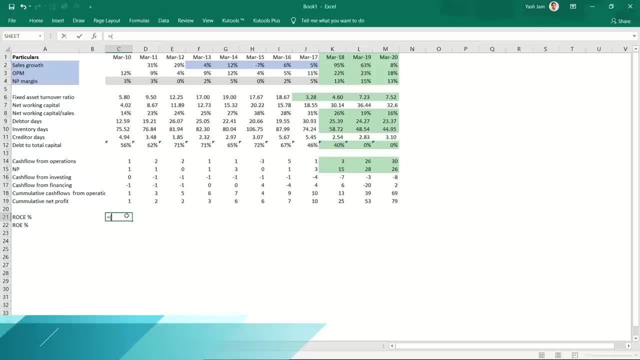 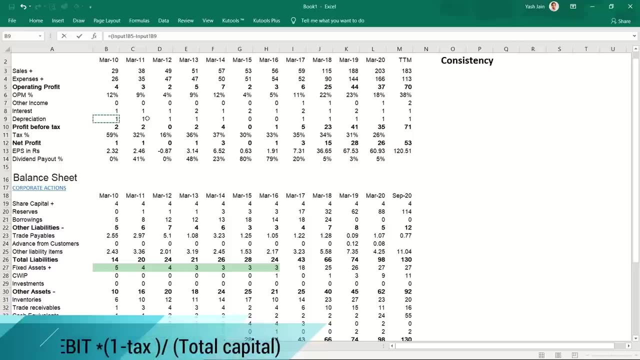 So you can do here: return on capital employed will be your operating profit, That is your EBITDA minus your depreciation. So that will be earning before interest in tax divided by- or maybe let's do it post tax- 1 minus rate of tax. 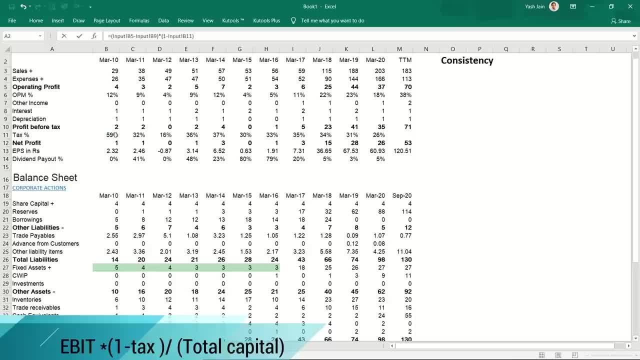 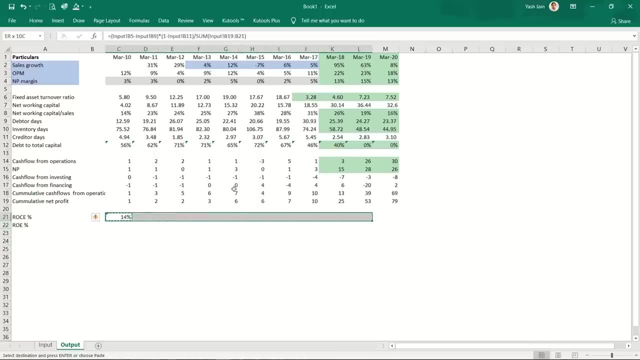 This is post tax earnings right From operations divided by total capital invested in the business, that is, share capital, reserves and borrowings. Okay, so it comes around 14%. Let me copy this and paste it. It could always be more than 20%. 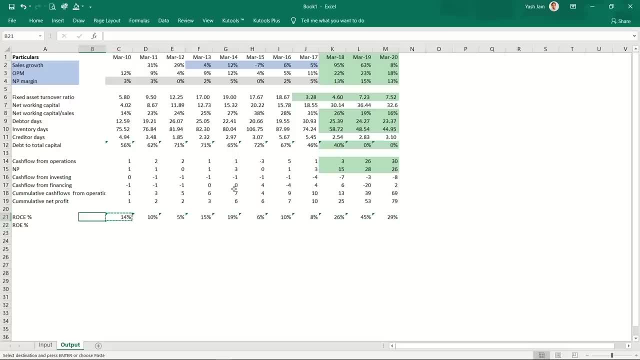 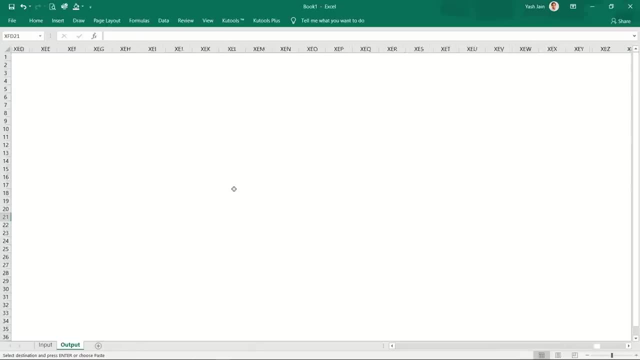 Okay, And don't forget that it should be in a growing trend or a stable trend. I can see here it was 14%, 10%, 5%, then again increase, so very unstable and revolving around 10 to 15% then, I think from here onwards. 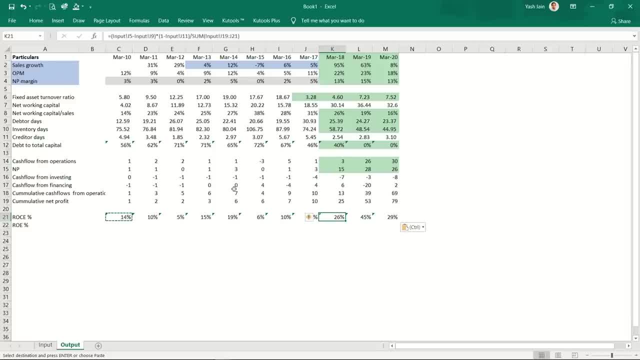 it started to increase, but since I think 2018, because they have paid majority of the debt, whatever profits are left are for equity holders. that's pretty good for 2018, 2019 and 2020, though this is bit concerning, it's bit unstable right: 26%, 45%, 29%, but I think as and when, 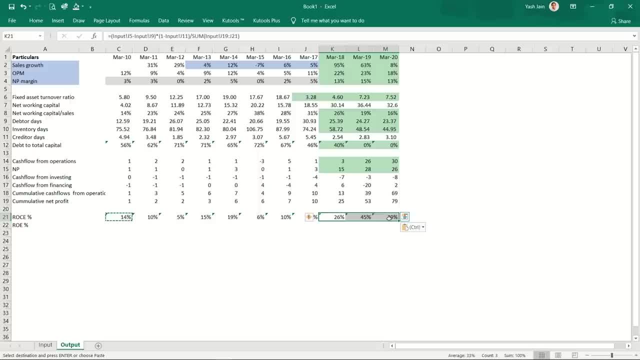 company matures: from small cap it moves towards mid cap and large cap. this will stabilize over the period, so this is also pretty positive for me. then return on equity. that is how much equity holders are generating, Not the only one, Not all the providers of capital, but just equity holders. so that will be net profit. 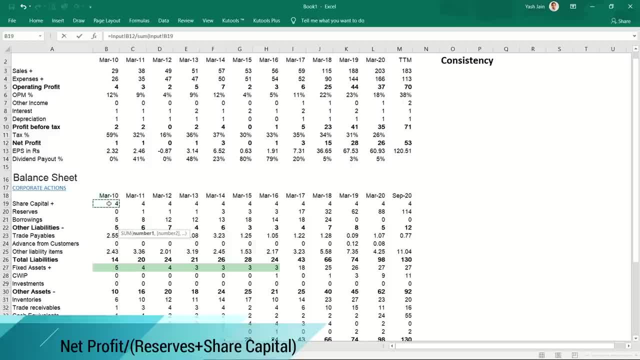 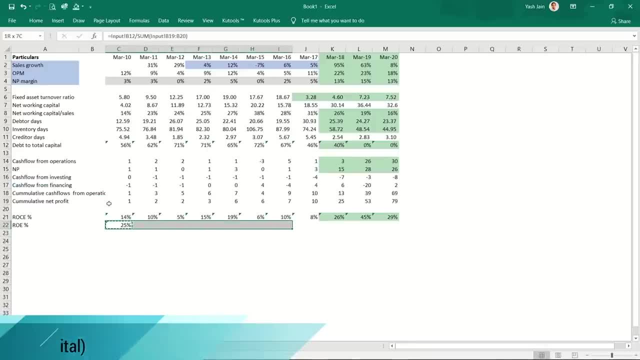 divided by equity invested in the business, that is, your share capital and retained earnings. you don't need to do this after tax because your net profits are already after tax. so you can see here it's pretty good from last 2-3 years. before that it was a bit like fluctuating. 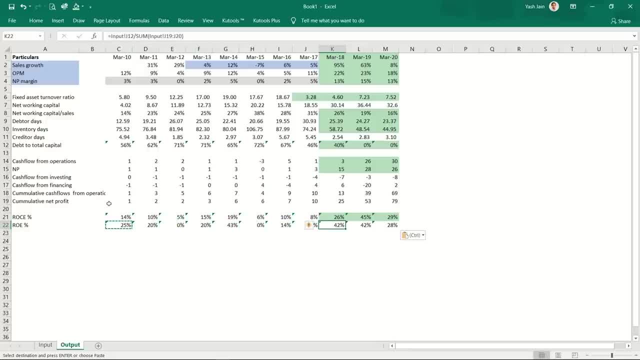 from 25% to 0%, then 43%, but I think company is becoming more stable in last 2-3 years. so that was it for my financial analysis video. I hope you learned something new. the most important thing is still the consistency. consistency: if the company is growing, it should. 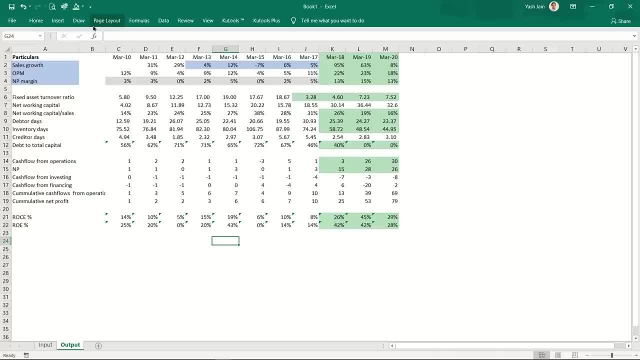 be growing consistently. if it is reducing its debt, it should be doing consistently. if profits are growing, it should be growing consistently. so everything should be very consistent, critical, stable In a company that you think would be doing very good going ahead in the future. so that's. 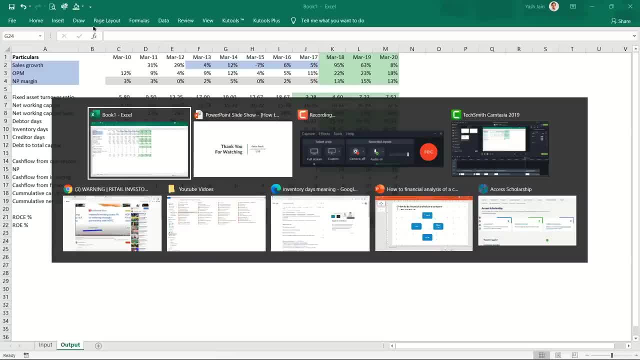 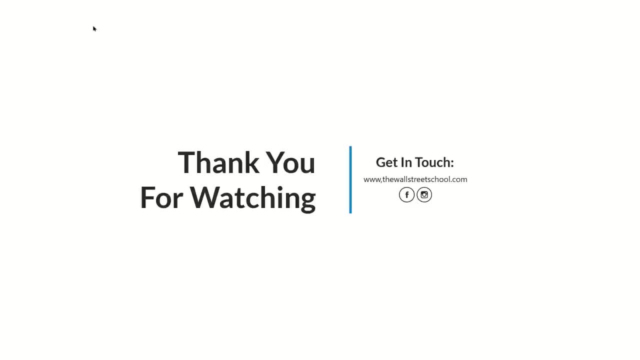 it for this video. if, in case, you have any doubts, feel free to reach us at the wallstreet school dot com or in the comment section below. I hope this video added some value to your time. thank you, bye, bye.